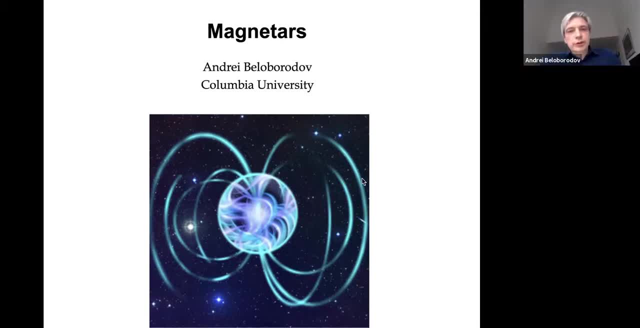 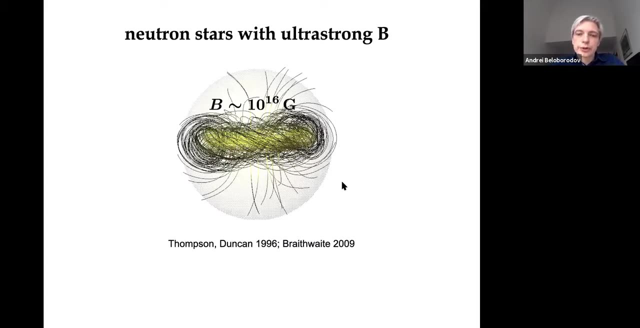 Go ahead. Okay, thank you for this introduction. My topic today is magnetars, And these are strongly magnetized neutron stars, stars. So I'll start with this little picture of a simulation that shows an initial state of the magnetic field in one model: how a Newton star is born with very strong magnetic. 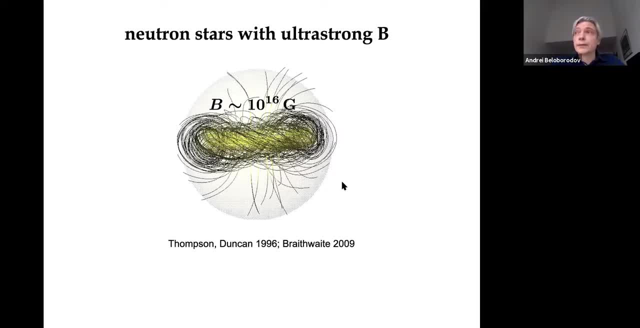 field up to 10 to the 16 counts. These strong fields end up from flux conservation as the star collapses, as the progenitor star collapses into a Newton star, compressing the magnetic flux with it, And in addition they can be dynamo mechanism that amplifies magnetic fields. 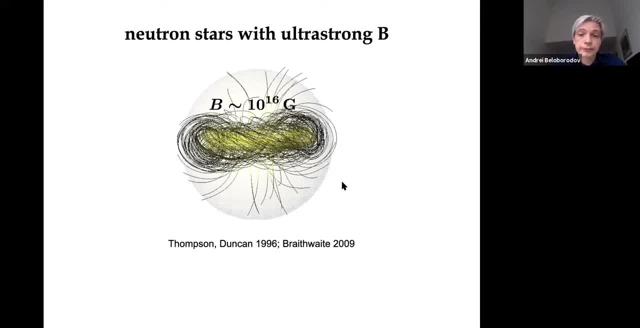 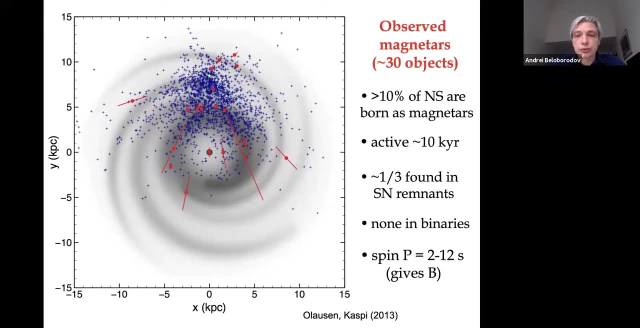 to up to 10, to the 16th, maybe even higher values. So we observe these ultra-magnetized Newton stars as very active X-ray sources. We know about 30 of them in our galaxy. This is the top view of our galaxy, the Milky Way. 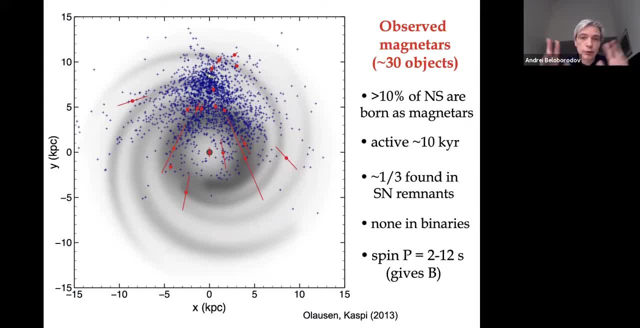 And you can see many blue crosses, which are ordinary Newton stars, normal radio pulses, And red symbols are magnetars. They are active, producing X-ray bursts and other stuff that I'll talk about later in my talk for about 10 kilo years, which is. 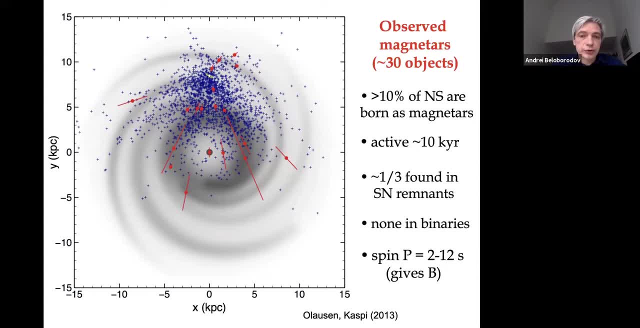 It's a small time compared to typical age of regular pulses, millions of years. So even though we don't see, We see only a few tens of them. in fact, at least 10%, maybe up to 50% of all Newton stars are born as magnetars. 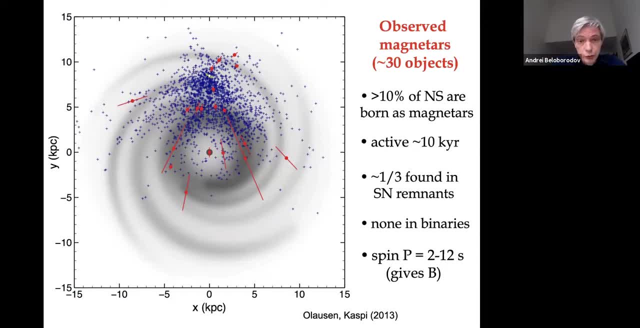 One third, about About one third, are found in supernova remnants. So we see that these objects are really products of stellar collapse. It also produces supernova explosion initially and then supernova remnants. Okay, None of them are found in binaries, So these are isolated objects. 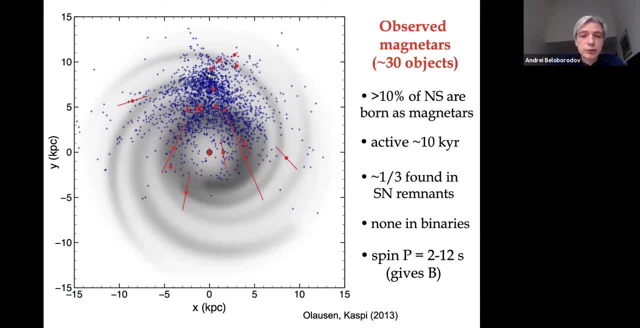 There are rotation periods that we observe are between 2 and 12 seconds, which is slow for their age And actually from the observed spin down rate we- It's one way of measuring magnetic fields- actually from the spin down rate of the Newton. 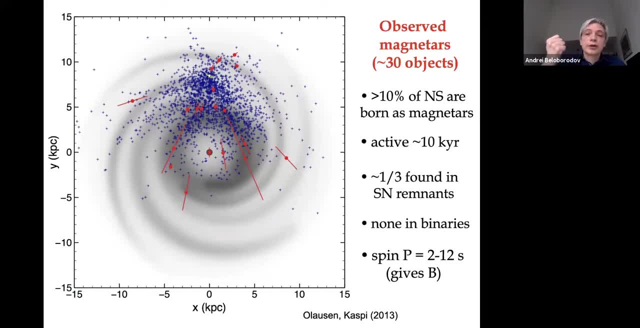 star. If you measure its period and time derivative of period, you can actually estimate the magnetic field. And this is how we can see that The fields go up to 10 to the 15th in the dipole component of the Newton star And we 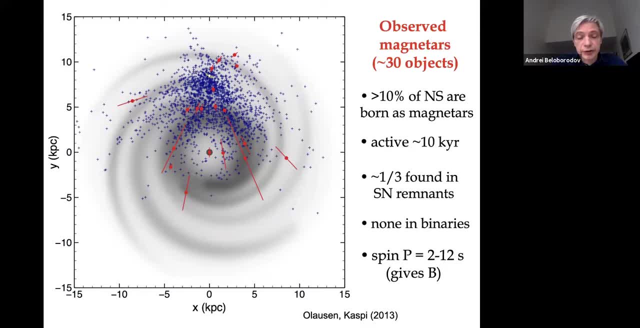 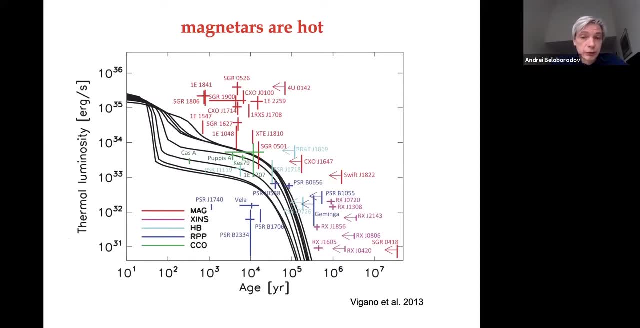 suspect even stronger fields inside the star, hidden inside the star for 10 to the 16th curves. Okay, These objects are very hot, unusually hot, You see here. Well, it's a busy plot, but basically you see many different, A few different classes of Newton stars and 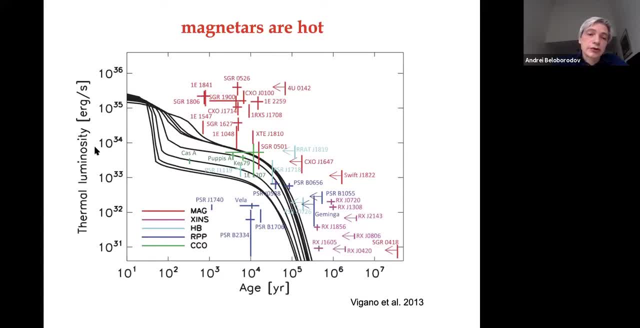 magnetars are shown here, Okay, And you can see here, you can see the red symbols, And so we can see the thermal luminosity of the surface temperature, if you like. Thermal luminosity scales as temperature to the fourth. The surface luminosity exceeds 10 to the 35 per second in some cases, And 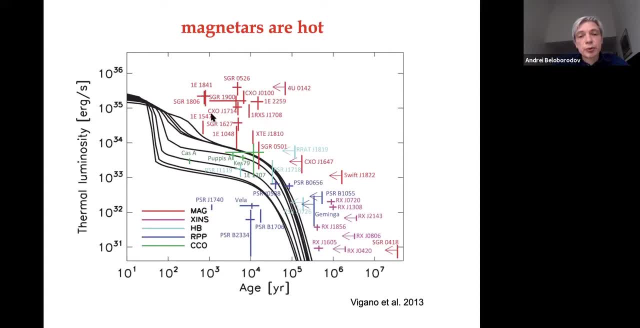 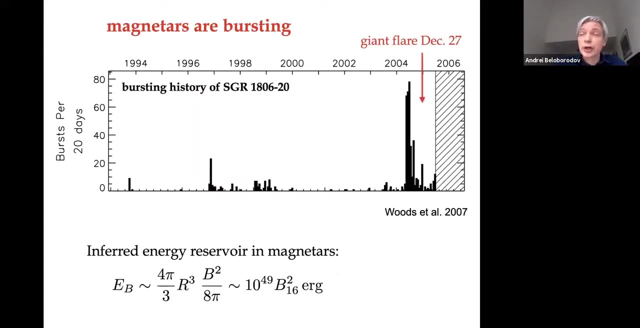 so all these red data points lie above other known, typical, you know, Newton stars in supernova, remnants And also Okay, So they are hot, They are also bursting. That's a remarkable feature And that's how mostly we discover them. now These magnetars are producing X-ray bursts. Typical duration: 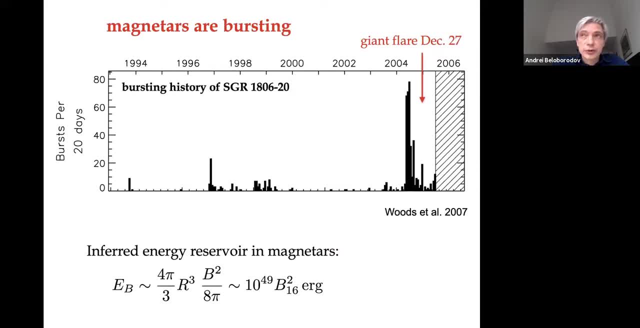 of an X-ray burst is about 0.1 second, And luminosity can go, for regular bursts, up to 10 to the 42 hertz per second, And sometimes these objects produce giant flares with luminosities up to 10 to the 47 hertz per second. For comparison, the luminosity of the Sun is 4 times 10 to the. 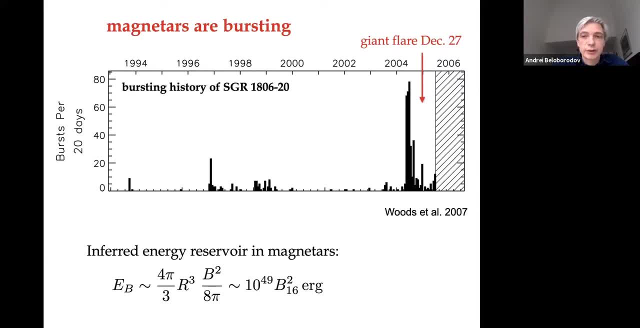 33 hertz per second, So these are tremendously bright objects And from this output that we observed you can estimate the total energy budget that you need over the lifetime. And then you find a number immediate in X-rays, something like 10 to the 48 perg, And 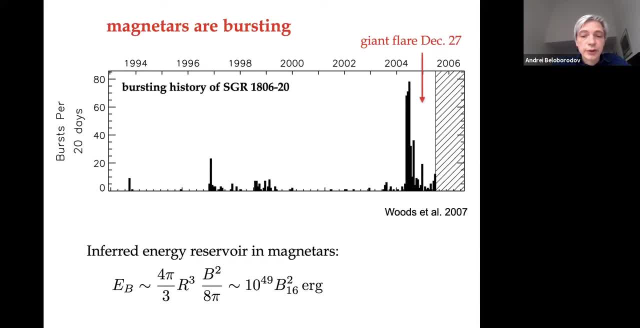 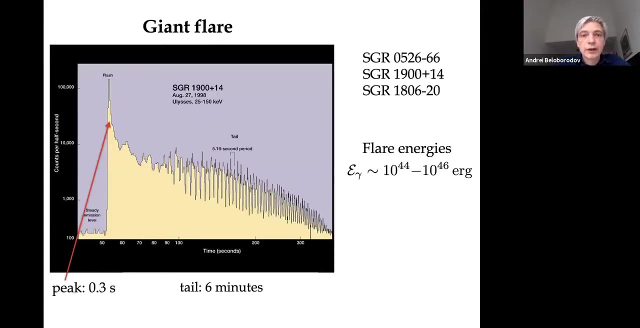 Assuming reasonable efficiency of- I'll talk a little bit about this later- You can conclude that about 10 to the 49, maybe 10 to the 50, is hidden inside the Newton star in the form of magnetic energy that feeds that earth activity. This is just one slide. 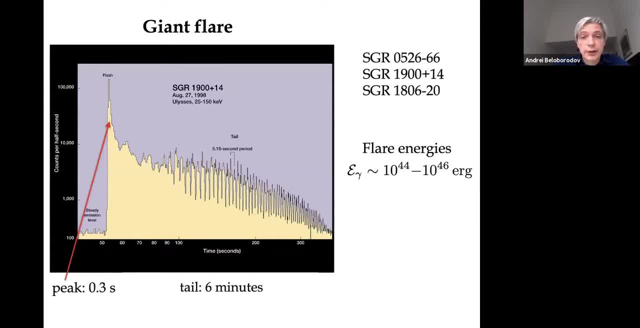 to show how remarkable the giant flares are. Basically, these are luminos. Well, luminosity is 10 to the 47 hertz per second. Total energy needed during the main peak of the flare and its oscillating tail can go up to 10 to the 46 hertz. The peak lasts a few tenths. 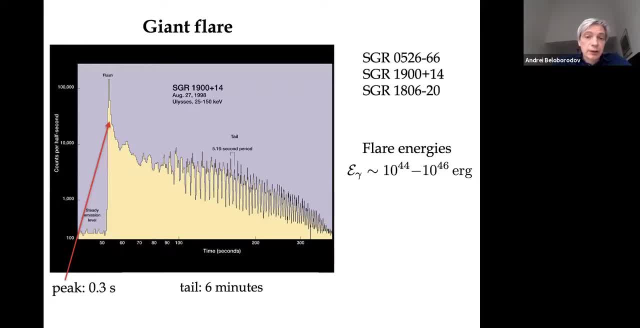 of a second and the tail goes for six minutes And we see about the same structure of the giant flare in three different flares observed by now. giant flares- Another interesting observational aspect, This really brief review of terminology of magnetars During the flare: periodic, quasi-periodic. 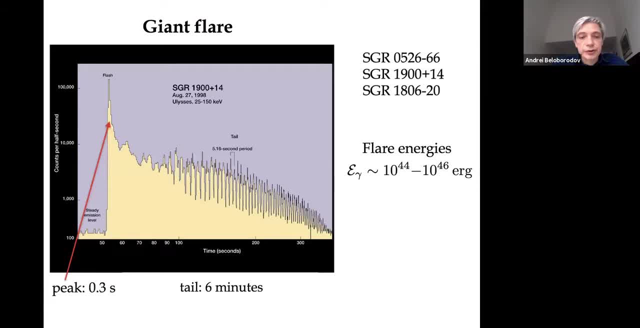 oscillations have been detected, high-frequency oscillations up to kilohertz range. So you can see this Fourier spectrum, So you can see peaks here which represent quasi-periodic oscillations, And the theoretical picture of these oscillations is on the right. 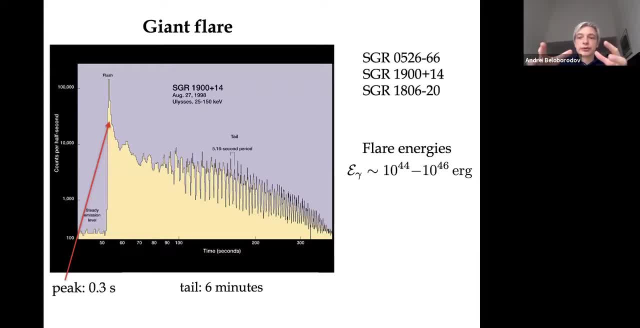 So the star is excited during the giant flare and it begins to oscillate. And by analyzing, by comparing the observed quasi-periodic oscillations with the theoretical models, it was concluded that there should be a superfluid neutron core inside the star. Well, we know that neutron 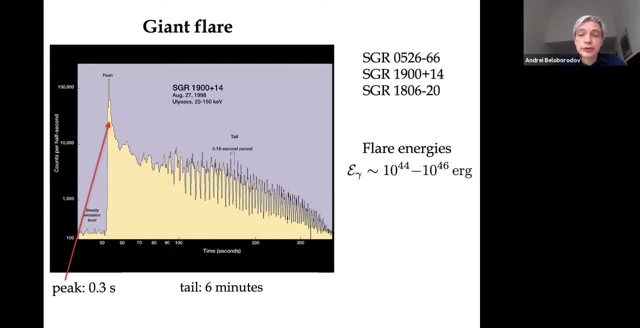 stars contain neutron cores. That's why they are called neutron stars. But also you can conclude that magnetars and more generally, neutral stars which are not too hot are superfluid. and this fact is actually was deduced also from from this quasi-partic oscillation, simply because when 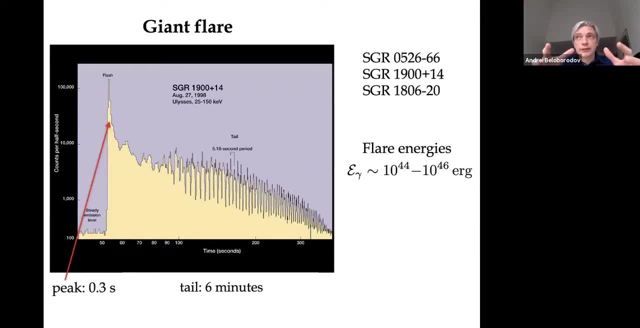 the star oscillates. its magnetic field, its plasma component, electron protein component are coupled together. they oscillate, but the neutrons, because they're superfluid, they're decoupled and don't contribute to the effective oscillating mass. that's how you can see this in the analysis of 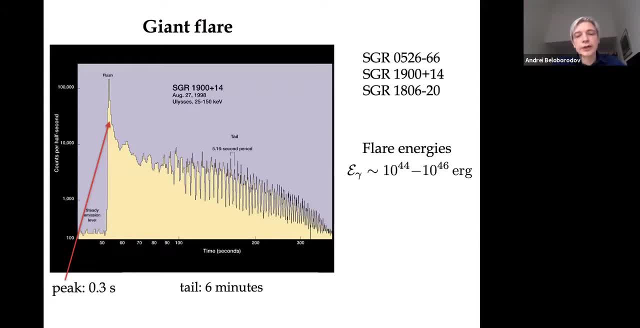 kpops, quasi-partic oscillations, all right. so the basic feature of magnetars is there is a lot of magnetic energy caged in the newton star, simply because neutron stars, even though they're called different neutron stars, they're excellent conductors. there is enough plasma and 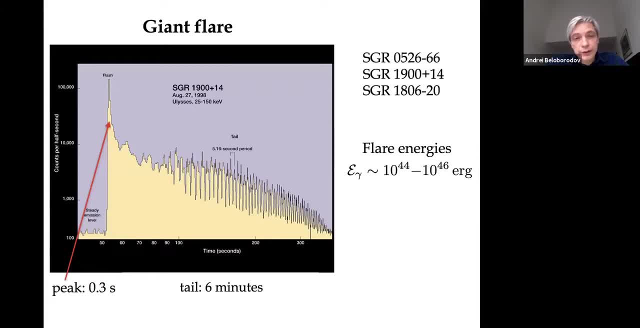 it's a very conducting medium, both core and the crust of the newton star, and so magnetic energy is trapped, magnetic field is frozen into this excellent conduct and, if you want, like a brief summary of the story of magnetars, the main drama is basically the desire of the magnetic. 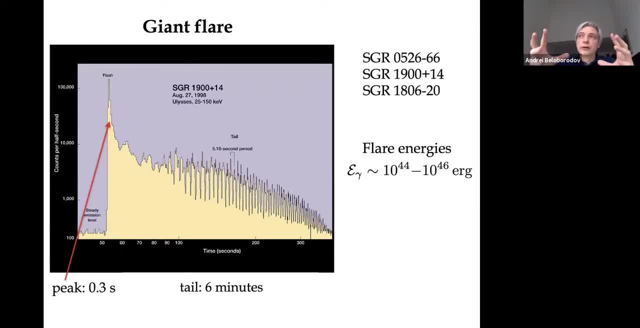 energy to get out from the star. if you imagine for a second that the star is not there, annihilated. what would the magnetic energy do? this 10 to the 50 euro? just explode, just expand. that's what electromagnetic field would like to do. but because it is frozen into this heavy conducting medium. 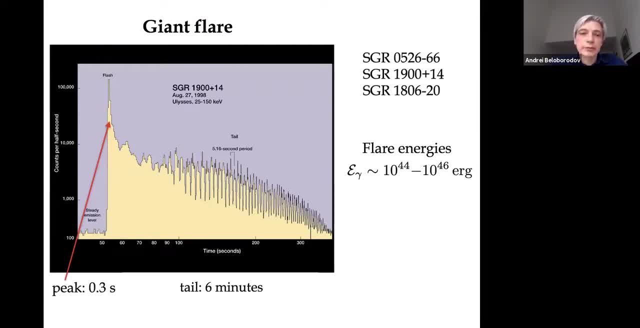 it stays there and it finds its way out gradually and slowly. it has to be sly and tricky to get out and there are a few uh stages of getting out, so i will discuss them in terms. so there is a core, some interesting dynamics is happening, there is a crust of the star. 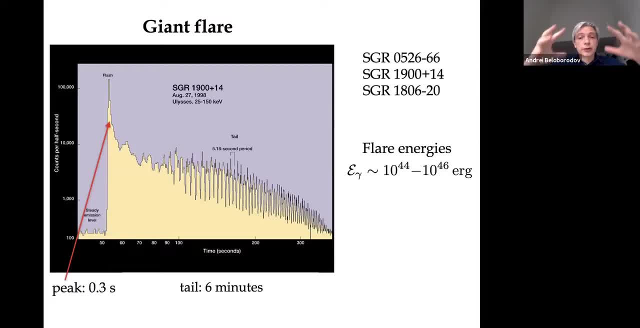 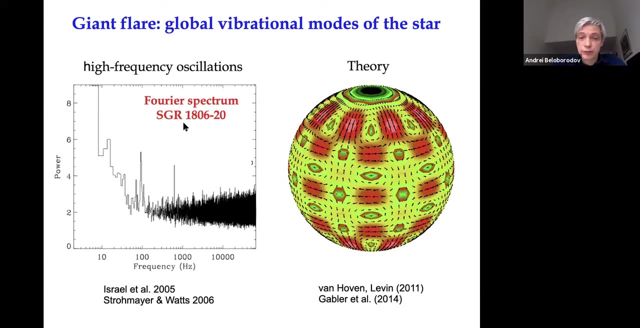 there is a magnetosphere around the star, so we need a sphere. and then there is a wind. okay, so let's start with the core. okay, so this slide that showed how quasi periodic oscillations are observed on the left and how theoretical models predict these oscillations on the right. okay, so i talked about 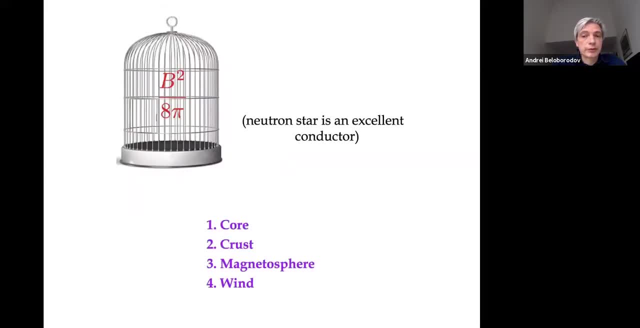 inferring that the core is super fluid from comparing theory observations. this little image can you see now slide switching: okay, and i'm on the next slide now. yes, okay, so you see the little cage and there is magnetic energy. yes, good, so So the magnetic field is really re-caged. 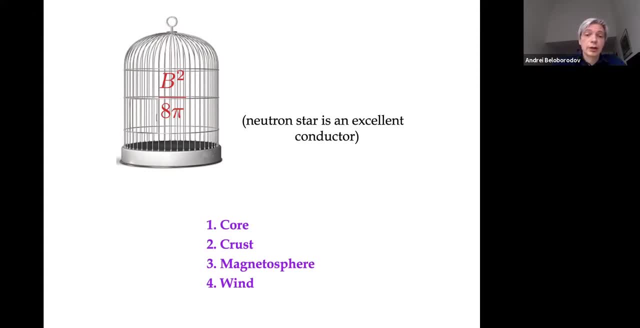 and it tries to get out. That's what I tried to explain And if it happens again, Igor, if you can just let me know, we'll do this again, because I don't know what's happening with Zoom, Absolutely Okay. 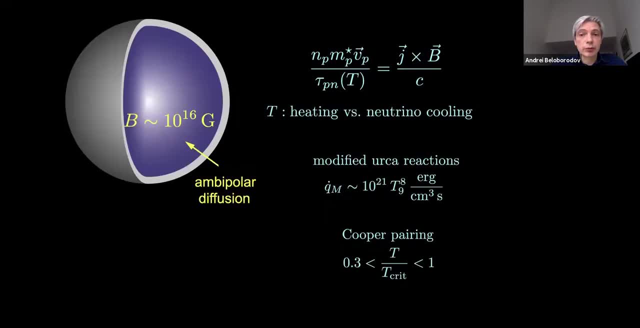 Nice, Okay, So let's move on then. So I would like to talk about the core and the basic process. there is ambipolar diffusion, So, okay, The star is born very hot- 10 to 11 Kelvin temperature- And it behaves as a single fluid initially. 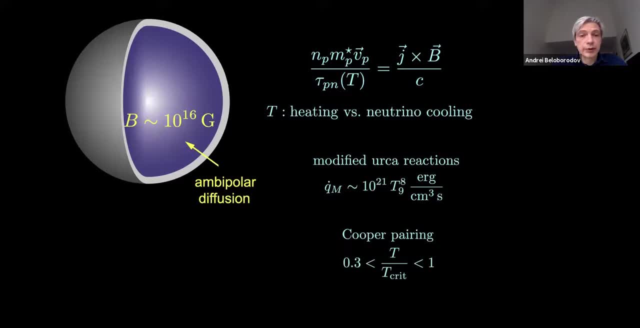 Nutrients and protons are colliding very frequently. They all couple together. Magnetic field is coupled to electron-proton component. However, later the star cools down and the very degenerate stuff that forms electrons, neutrons and protons. 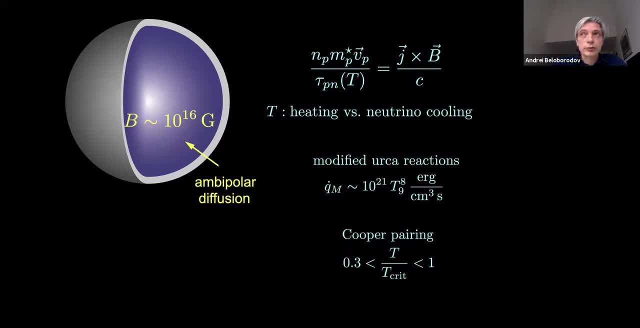 because it's degenerate particles, particularly neutrons and protons, collide much less frequently. The free path of particles. degenerate particles come, becomes large And now electrons and protons would like, can move with respect to neutrons with some rate. 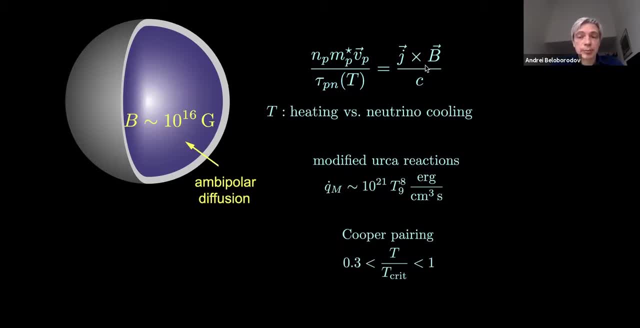 Now the reason why they would like to move. there is a, J cross, B force, The amper force. Of course there is J in the star because there is B. J is the current density, B is the magnetic field. So you cannot have a force-free configuration there. 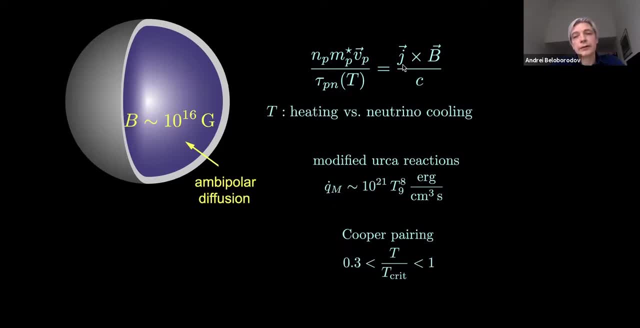 So there is a component of J cross B, that product of current and magnetic field, And this is the force that would like to move the magnetic field- essentially magnetic field and plasma, Out of the star. eventually, There is also a force that imposes that, the frictional force. 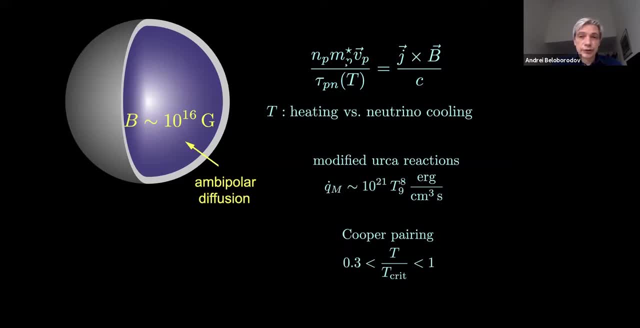 that electrons and protons are colliding with neutrons, And so the result: there is a force balance between the friction and the amper force. J cross B. As I said already, the time scale for proton-neutron collision depends on temperature. 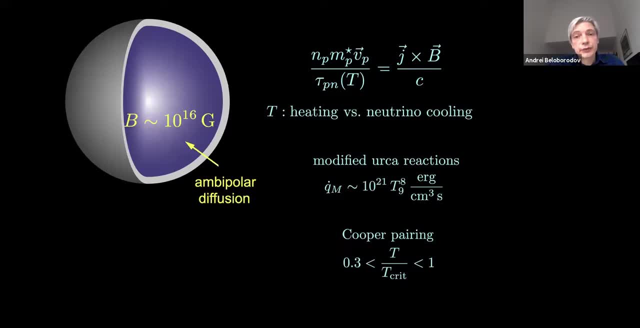 And therefore the balance. this equation, which determines the velocity of the electron-proton fluid And therefore the velocity of the magnetic field lines with the aside, works together with the electron-proton fluid. This velocity depends on temperature of the star. In turn, temperatures controlled. 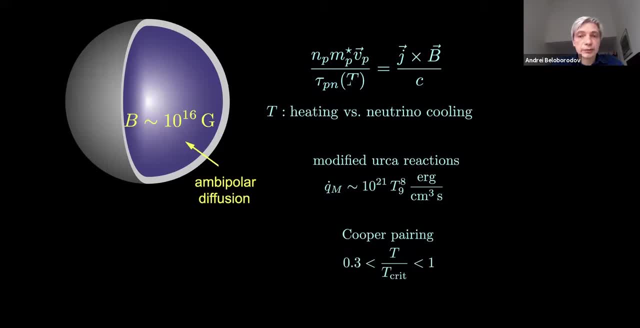 by the balance between heating which comes from ampli polar diffusion. This frictional force is a dissipative results and dissipation. So there is heating release, biometric antipolar diffusion, So this big process is called antipolar diffusion. 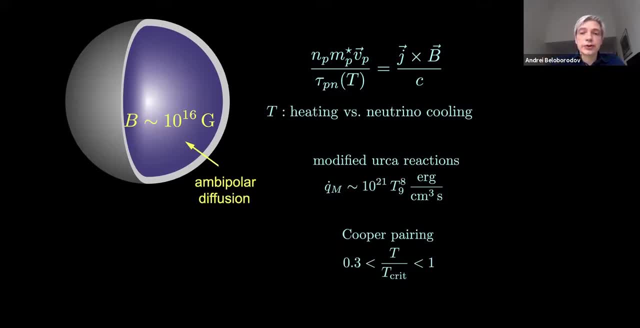 It produces heat. On the other hand, the core is cooled by neutrino emission And the main cooling process is a so-called modified Ulker reactions. So there is direct Ulker reactions when electrons combine with protons into neutrons and neutrino. 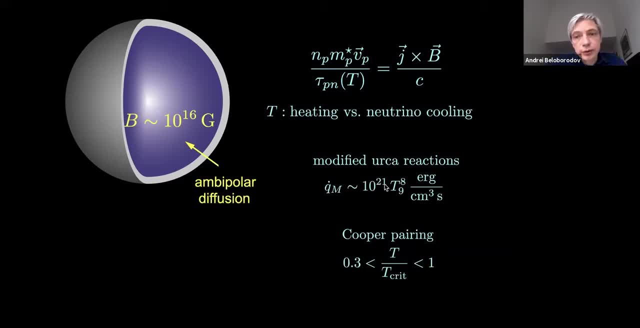 And then there is the opposite process of decay of neutron and proton and electron, And so when these processes happen frequently they steal energy. it's called Ulker reaction. So modified Ulker is similar, but it involves another particle. It becomes free body reaction spectator-nuclein. 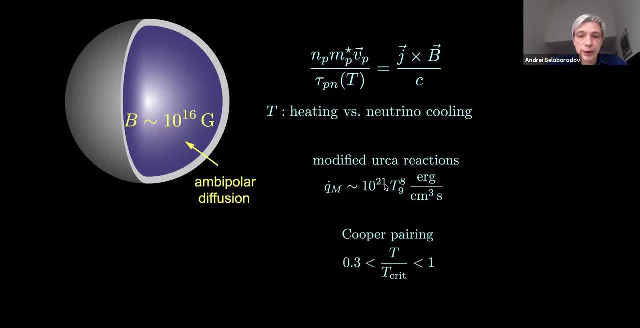 which can take the excess of momentum when direct Ulker is prohibited because there is an energy gap for direct Ulker, So anyway. so this is the process which is very sensitive to temperature of the Newton star And it can be very efficient, cooler at high temperatures. 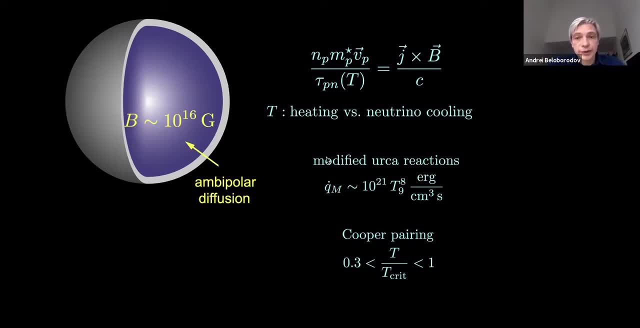 when the star is young. Okay, so that's what's happening. basically, The star is cooled by neutrinos and it's heated by antipolar diffusion. There is an additional cooling process which becomes important. when the star goes through the, its temperature drops below the critical temperature. 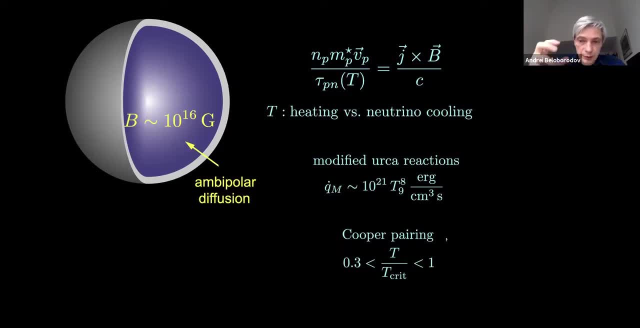 So cool, preparing of inference, So then it becomes super fluid but it takes some range of temperatures and cool prepares form and reform and producing neutrinos. and I can try to do during the state when the temperature is between 0.3 and one of the critical temperature. 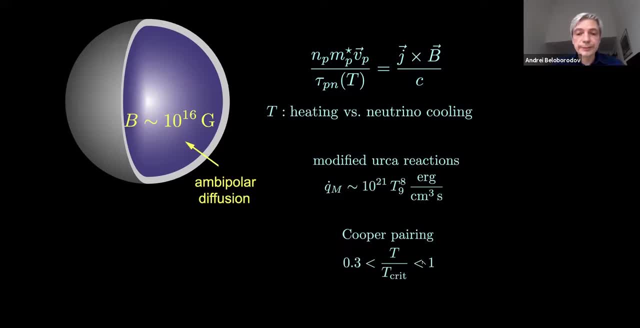 So actually during this transition the cooling rate is enhanced. So anyway, so this process are relatively well understood And one can estimate that estimate, the thermal evolution of the star, And basically we're dealing here with a couple problem of how the star is heated by MPO diffusion and cooled. 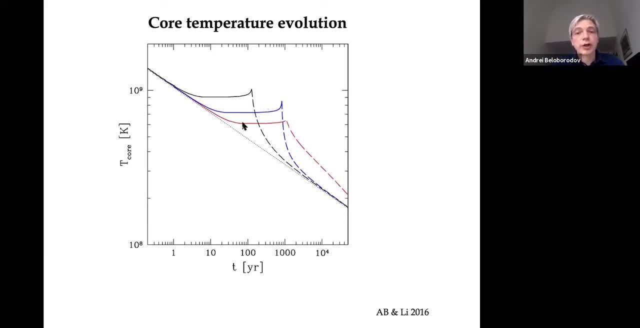 And the self consistent evolution here can be estimated as Paul chose. the result with just modified hooker reactions without super fluidity, And the characteristic temperature is about 10 to the ninth Kelvin, a little bit below it, very hot core. The dotted line shows what would happen. 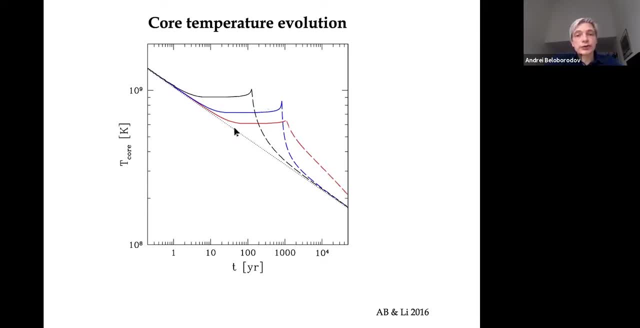 if there are no MPO diffusion, The temperature of the star would just cool down. When MPO diffusion switches on, the magnetic energy converts to heat partially and offsets neutrino cooling, And for a while, for centuries. actually there is a balance between MPO diffusion. 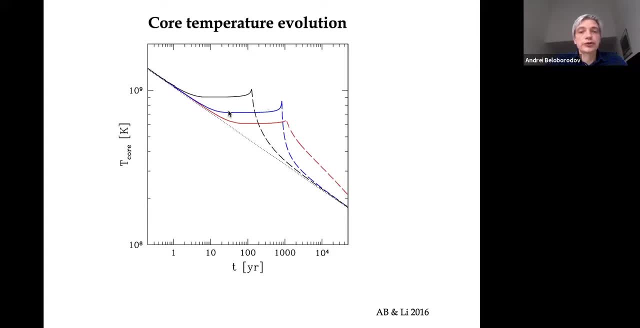 heating and neutrino cooling. Okay, so we see this white part And eventually it ends, and then MPO diffusion is choked and we have transitioned to super fluidity, et cetera. So this stage was roughly a thousand years, but actually I'll come back to this point. 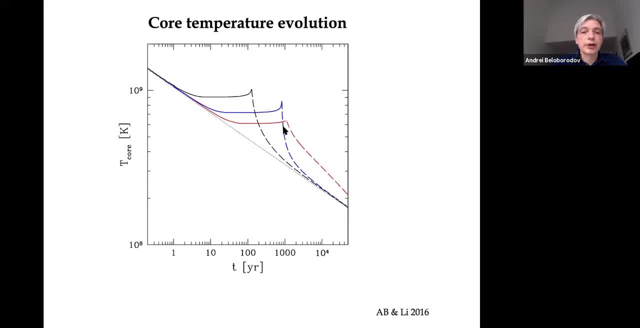 If the star is especially strongly magnetized, it can last only a few decades. And then it's. you expect a particularly violent MPO diffusion, And you can see that. You can see that here. the stronger is the diffusion, the stronger is the heating. 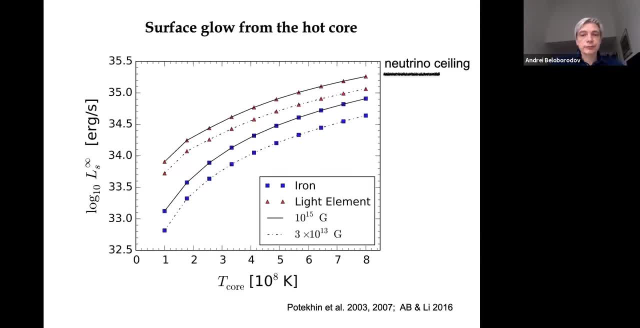 and the shorter is the lifetime of this process. Observationally, when you look at this object heated at the core, you get some heat diffusing to the surface. So most of the produced heat escapes in neutrinos. but because the core is hot, 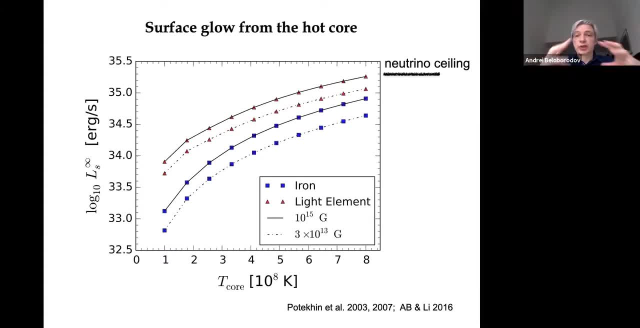 you also have heat conduction, And on a timescale of several months the heat reaches the surface and establishes quasi steady state. So this is what we call thermal conduction. The thermal conductivity is lowest in the upper layers of the crust, And so it's like a blanket around the star. 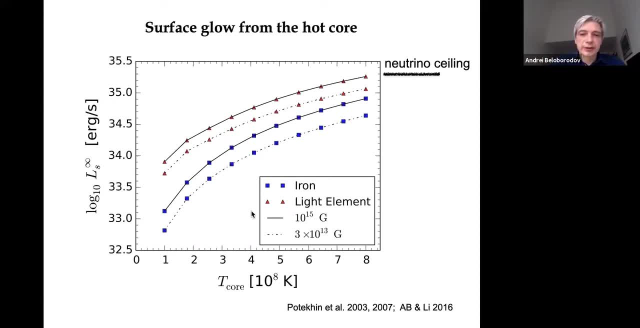 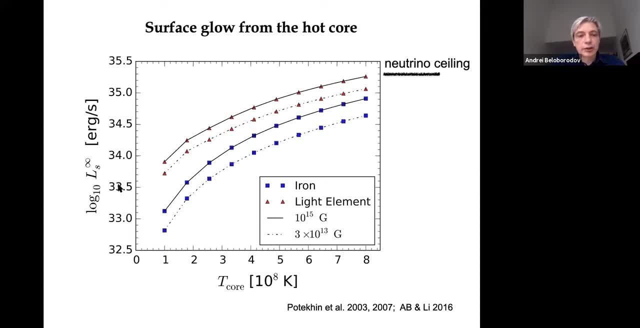 the internal temperature of the star and its thermal luminosity from the surface. depending on the composition of this blanket- it could be pure iron or it could be some, could be some light elements- you get some different results, but the bottom line is that you find 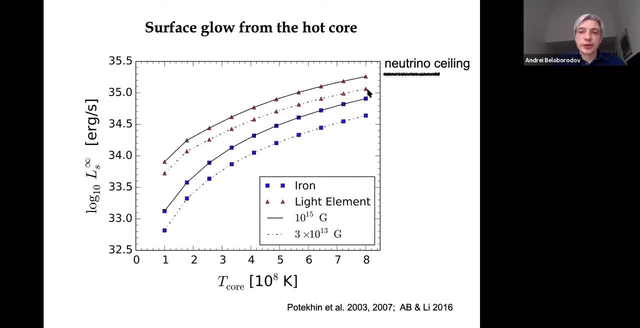 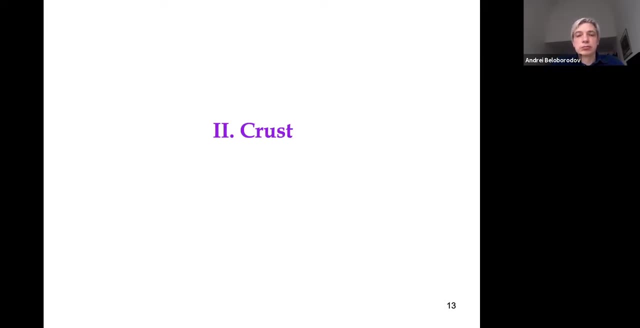 that the surface temperature is comparable to 10 to the sixth Kelvin, while the internal temperature varies between 10 to the eighth and 10 to the ninth. Okay, So that's what comes out from from ambipolar diffusion. There's the magnetic field tries to get out from the core, dissipates a lot of energy on the way. 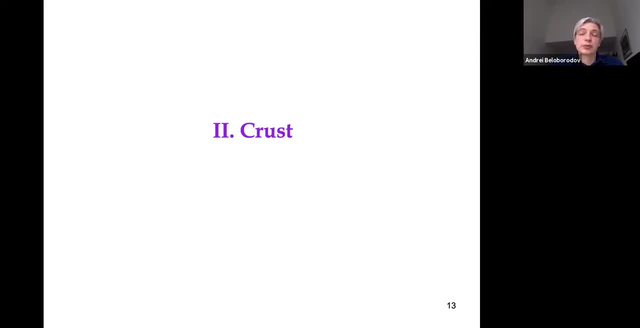 most of it goes into neutrinos and some of them, a small fraction, reaches the surface and you see emission from the surface, thermal emission. Now what's happening in the crust? In the crust, the magnetic field lines can also evolve because of the process that is called. 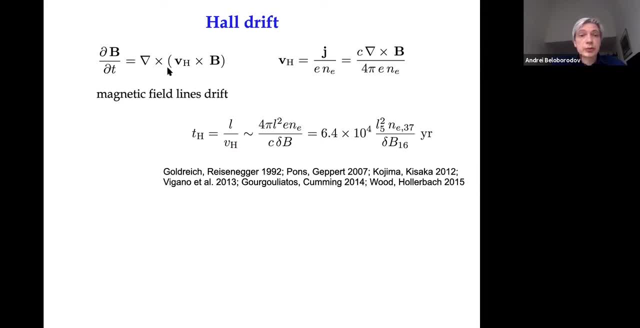 hold drift. Summarized by the simple equation, it basically states that magnetic field lines are frozen into electron fluid. So if there are electric currents flowing in the crust, use current density j. you have some electron density- m, e- which we know- in the crust. 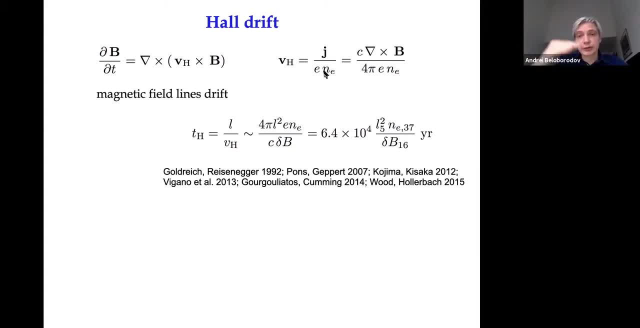 we know all the properties of interest rate, density, stratification, etc. And so the h is this so whole velocity of electrons? The electrons have very low mass and therefore their rest frame, electric field, should be zero. That's the condition. that is basically telling you. 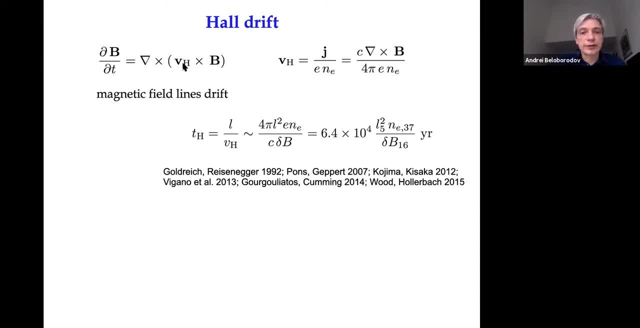 that db, dt, which we know is negative, curl e right induction equation. So this electric field in the lock frame is found from the condition that the electric field in the rest frame of the drifting electrons is zero. So e is negative, e whole times b. Okay, so this is basically induction. 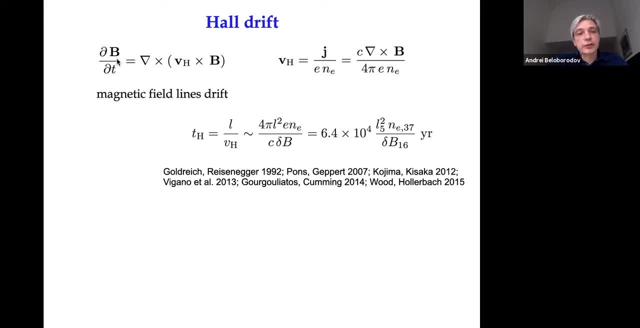 equation. On the other hand, this equation states that b is frozen into the electron fluid, which may be moving with some image. So magnetic fields are being deformed. They follow the motion of the electron fluid through the crust. The crust is a solid and therefore ions are static. 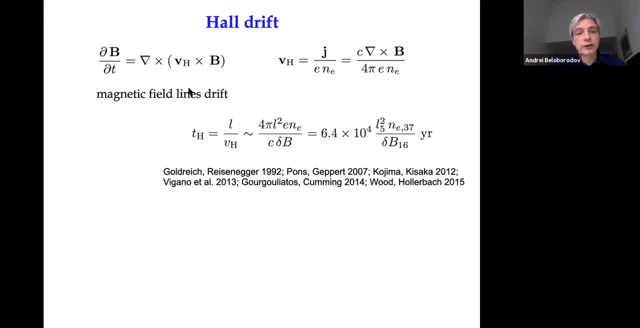 in the lattice and the electrons are drifting through the crust. The time scale for this process can be easily estimated from these equations and, depending on the strength of the magnetic field and the scale of variation of b and the crust, can be 10 to the 4 years, relatively slow. 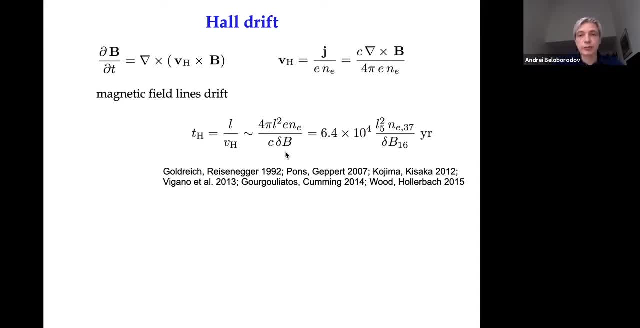 process Very well studied, especially in recent years, probably in three-dimensional simulations. There is also such a thing as whole waves. It's a simple example of this whole grid. So when you imagine a radiation problem, you have a vertical field in the z direction. 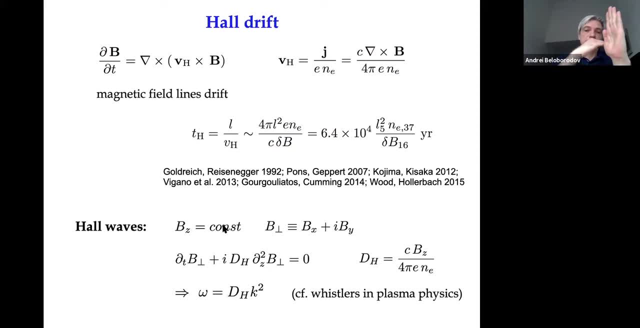 Horizontal plane is parallel to the, let's say, the surface of the star And you look at how the perpendicular component of the magnetic field evolves in time. it's easy to derive. you know equations for this problem And then you will see that this system supports waves described by this equation here. 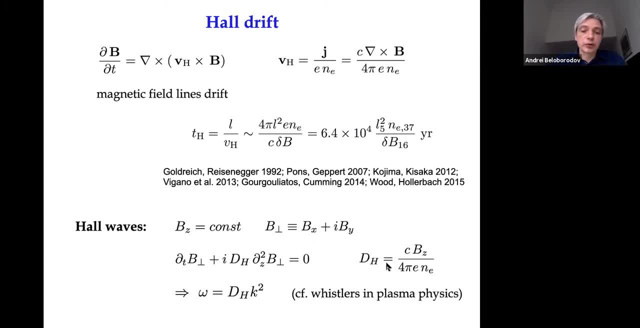 When capital D, H is the whole condition, so-called, which determines the dispersion relation for these waves. Because there is I. you see that the wave is going to rotate: The electric field, the, the magnetic field is going to rotate in this wave. 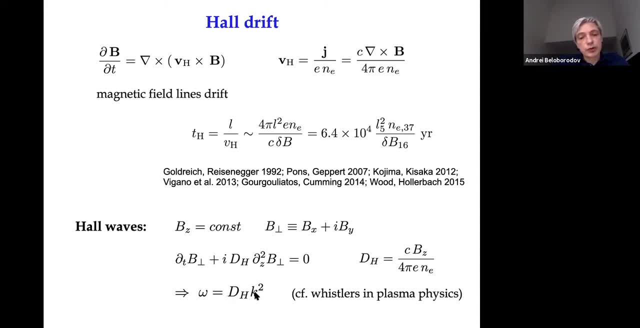 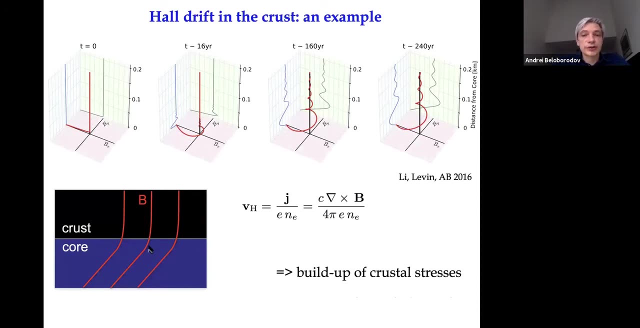 The dispersion relation also gives you the free speed omega over K, which grows with K. That means that the high K modes with high wave number modes are propagating fastest the school waves, fastest short wavelengths. Just to give you one simple example of how this process works in the crust. 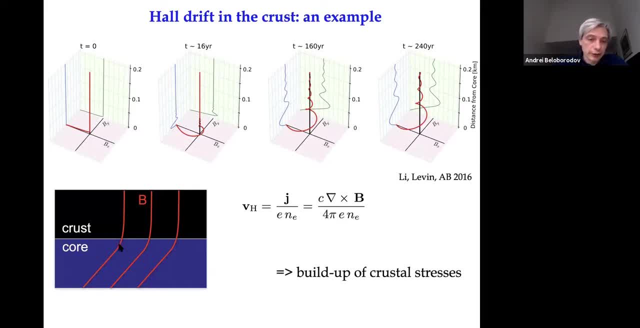 So imagine a liquid infant, like the problem core, and there is a boundary here above it to get crossed. And suppose, some people, diffusion has done it's some evolution of magnetic field. Well, the field is still frozen in the crust because it evolves in so long per time scale. 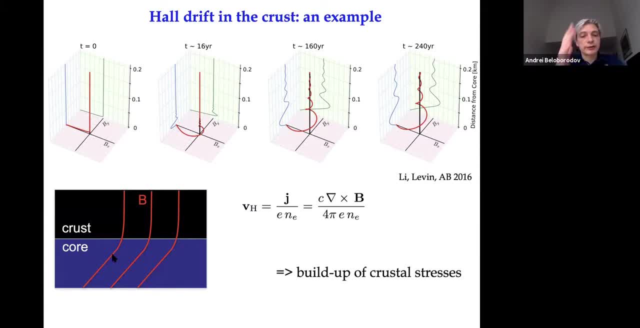 Then you create this kink in the magnetic field lines. The field now has a kink, which means that there is a current sheet here At the interface of the core of the crust, And this is the initial condition for launching, after this, fast and default diffusion phase. 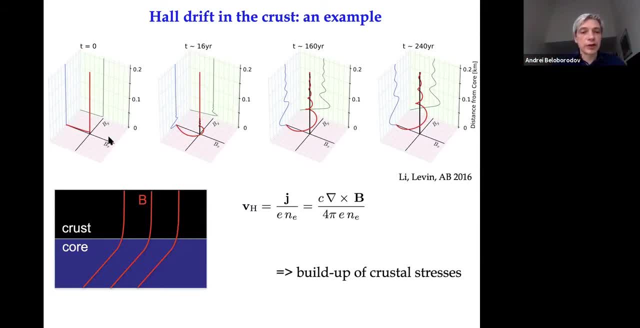 It sets the initial condition for launching whole waves into the crust And their panels here about show. this red curve shows that. well, you can think of it as an end point of the magnetic vector, this B curve. So initially it goes like this and there is no B curve. 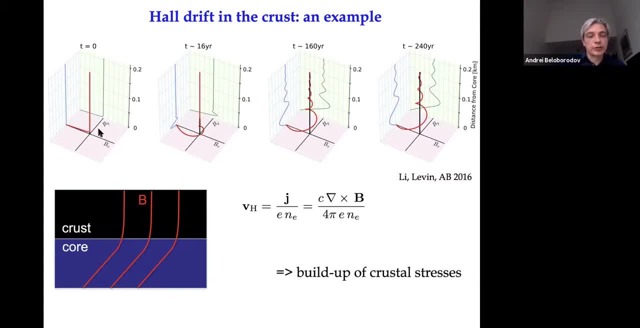 This is the end point of the wave in the crust. This pink plane is the interface of the crust and the core And as you let it go, this magnetic vector begins to rotate and grow. So you want you, this circle of propagating whole wave into the crust. 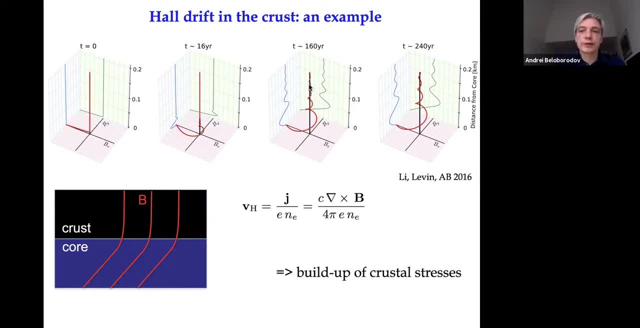 And, as you can see, the short wave wave is propagated ahead of the long wave. So it just a simple example of how you create magnetic field evolution in the crust. What you also find is that it generates stresses, magnetic stresses in the crust. 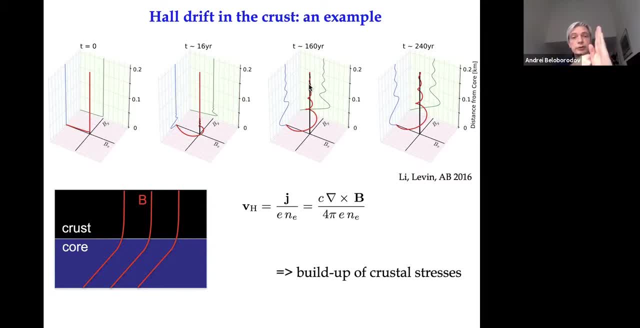 The product of BZ vertical field and B horizontal is the stress, magnetic stress- And this stress is applied to the solid crust. It's helped by the solid And at some point another thing can happen. The crust can yield to this stress mechanically. 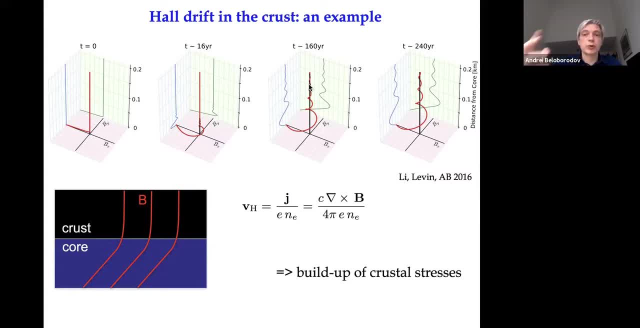 So the whole drift itself is dissipation. So it's very good, It's promising. The magnetic field has found the way of getting out, like diffusing its energy through the core up to the magnetosphere without losses. That's good, But on the other hand it does create small scale structure. 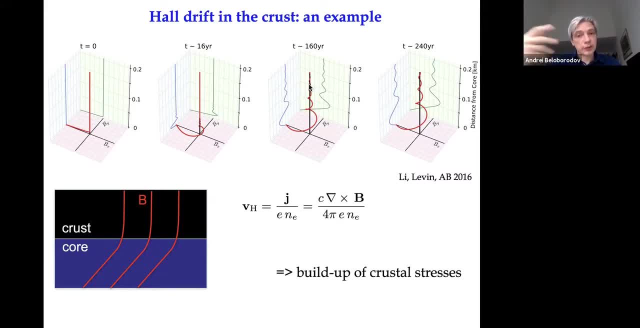 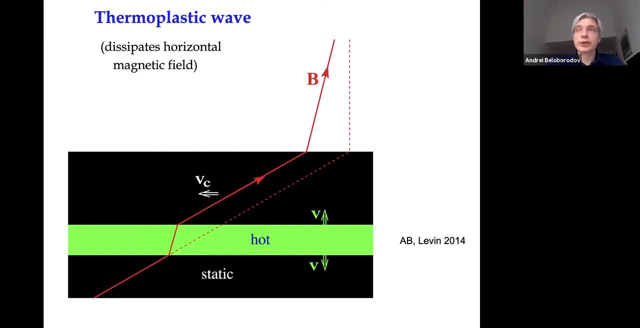 which can become prone to omic dissipation and the magnetic field begins to move its energy And it also can initiate mechanical failure. Just to explain quickly: this is not a basic building block of our lives, Just a simple mechanism, like basic mechanism, of how it can work. 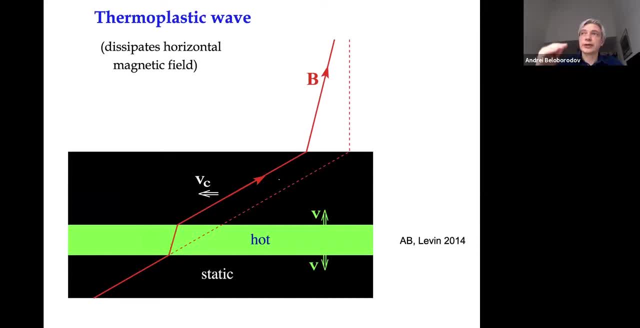 Imagine you have magnetic field threading the crust and it applies stress And at some point it becomes intolerable for the crust, meaning that the crust, the solid, yields in some layer. What happens then? The layer begins to flow plastically and plastic flows dissipate if you generate heat. 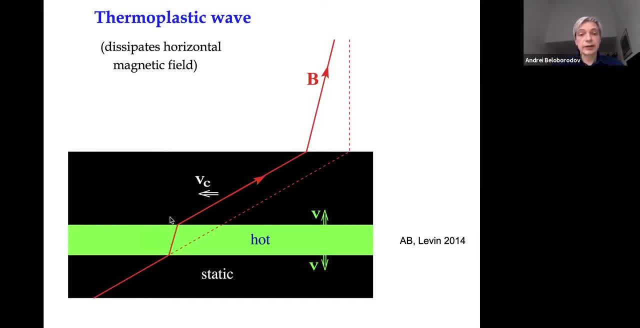 And then this heat begins to be conducted out of this layer And as the heat is conducted it softens the material and it continues to yield to magnetic stresses. And you want your wave. It's pretty much. it's very similar to deflagration wave. 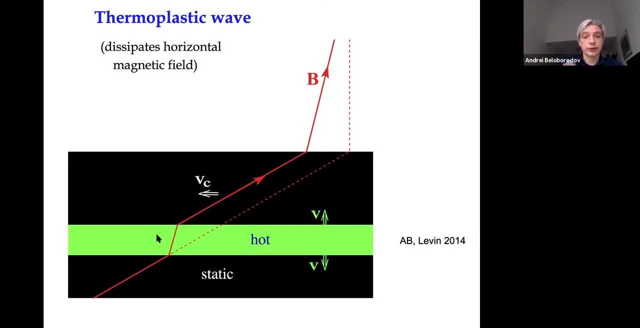 Like you use match to ignite fire and then you begin to use energy. Basically, it's a instead of chemical fluid fuel. it's a instead of chemical fluid fuel. we have here magnetic energy which is being burned. 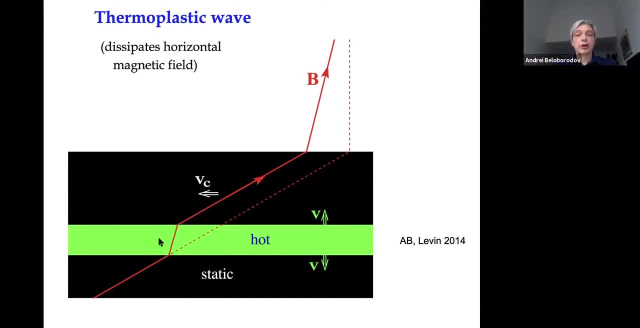 the horizontal component of magnetic energy, And then you launch a front which can dissipate this magnetic energy into heat. In extreme cases, when the field is strong, it can actually even melt the crust And this green zone becomes so hot that this layer is melted. 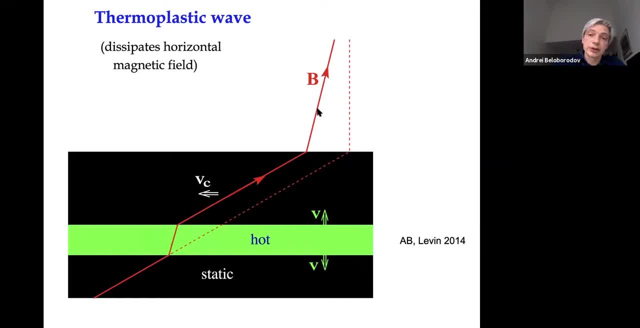 And of course it does. it allows this magnetic stress, like this fuel line, cools the upper slab and it allows the magnetic stress to cool And it allows the magnetic fuel to relax, to move over the core configuration here. So what happens in these waves is that you have motions. 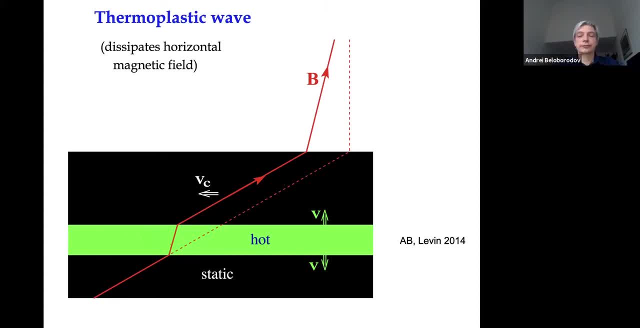 relative motion, horizontal motions in the past four years. So of course this weight, in this way magnetic field loses energy, dissipates energy, But part of it succeeds and gets out of the star because these motions of the plates deform the magnetic field, that the external magnetic field. 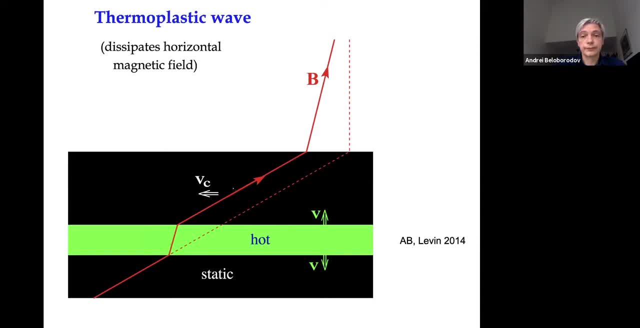 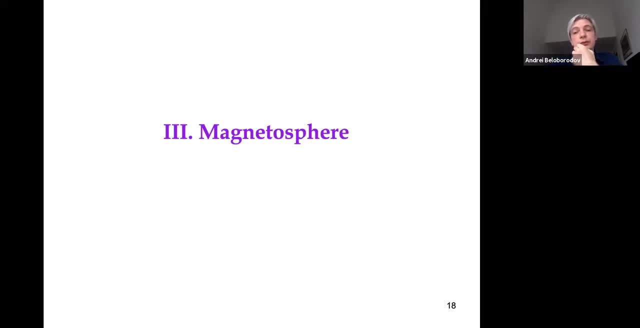 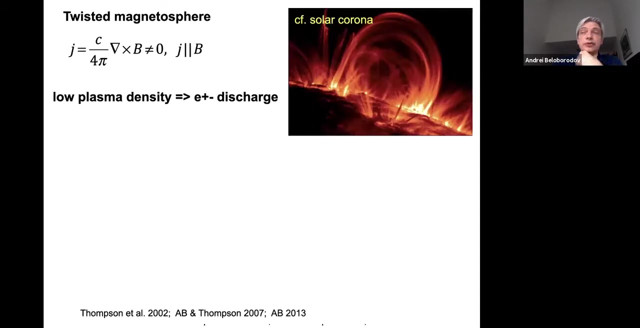 that is attached to the neutron star. All right, So now let me talk about what happens in the magnetosphere. So the magnetosphere is deformed by this surface motions- crustal motions of the magnetar- And as a result, it resembles solar corona. 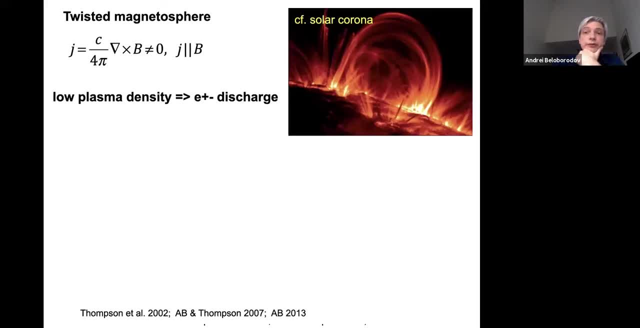 In the following sense: the field becomes twisted, deformed And it is pretty much force free, what they call, in the sense that J is parallel to B, The solar corona is magnetically dominated And also the magnetosphere of the neutron star. 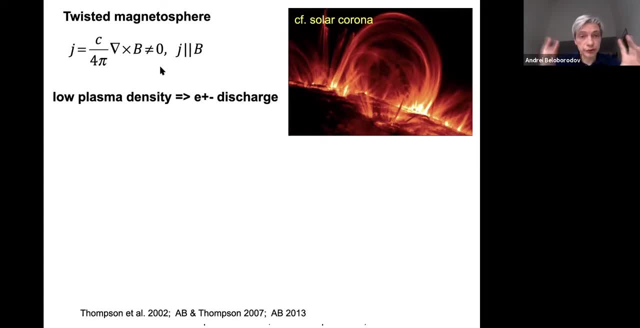 by definition, is probably magnetically dominated. Magnetic field is the dominant form of energy there. It's very strong. Whatever particles are living in the magnetosphere, they are sitting in the zero unbound level, So they move frequently along the magnetic field lines. 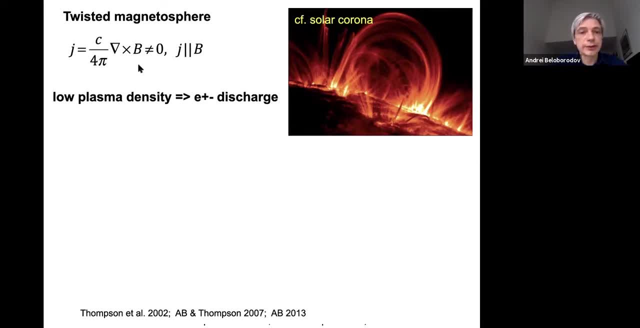 And then we try to excite the perpendicular motions right away, immediately, And so suppose you have twisted up this external field Before you do that? the magnetosphere. let's imagine a simple dipole configuration. It can be plasma free. 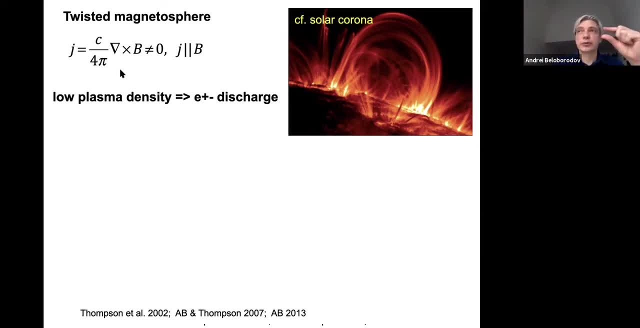 The hydrostatic scale height of the plasma layer on the surface can be plasma free. The hydrostatic scale height of the plasma layer on the surface. the radius of the neutron star is a few centimeters. One to 10 centimeters is tiny. compared to the radius of the neutron star, which is 10, 12 kilometers. So naively, you would say there is no plasma. There is exponentially reduced plasma density. However, it is a difference from the solar corona: We have plenty of plasma. 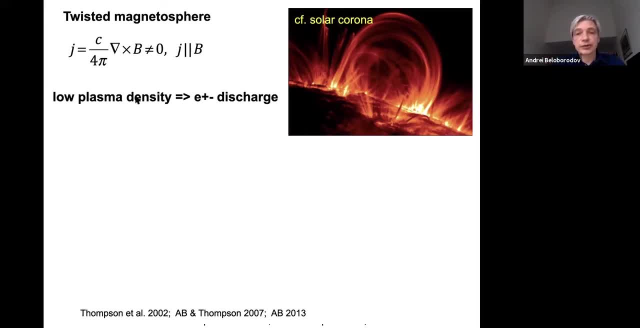 However, when you begin to twist the magnetic fields, you ignite the electron positional discharge which fills than with the sphere with plasma. The mechanism for this discharge is very straightforward. So you have, you begin to accelerate seed particle, So electric field begins to accelerate seed particles. 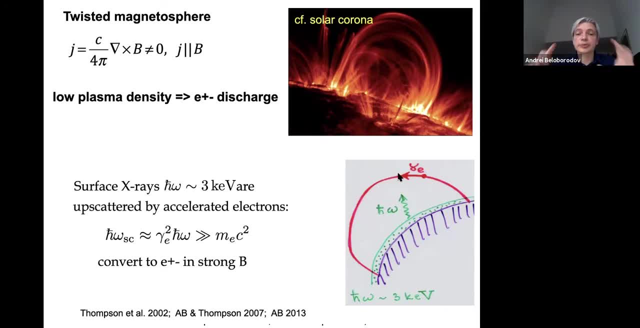 to higher tolerance factors And these seed particles upscale them. Whatever background photons are, this star emits KV photons, X-rays, And this particle can resonantly actually upscale these photons to this area. When this photon is more shifted to the breast from of the particle can find presence with the one down energy. 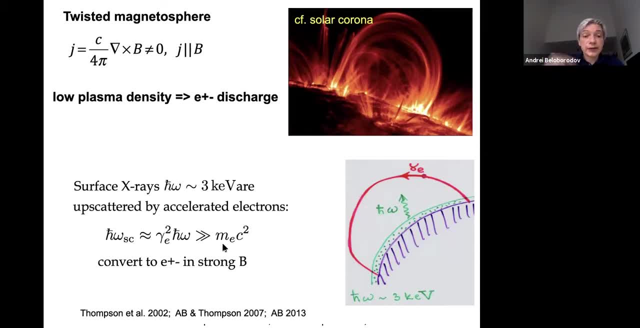 And then the cross-section of the scattering becomes big And this scattered photon gains energy. for gamma-squared, the electron tolerance factor squared And it can end up with energy much higher than the breast mass. Then this photon easily converts to a composting. here. 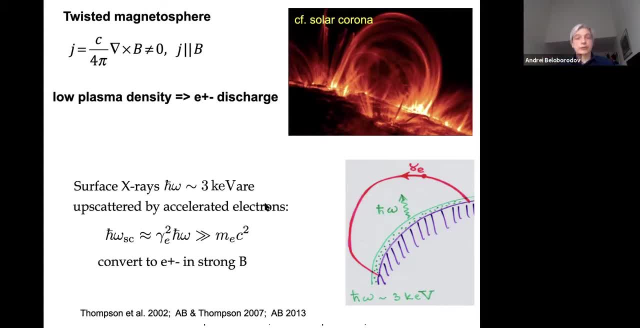 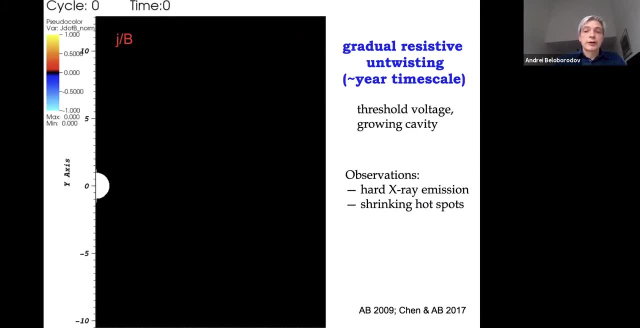 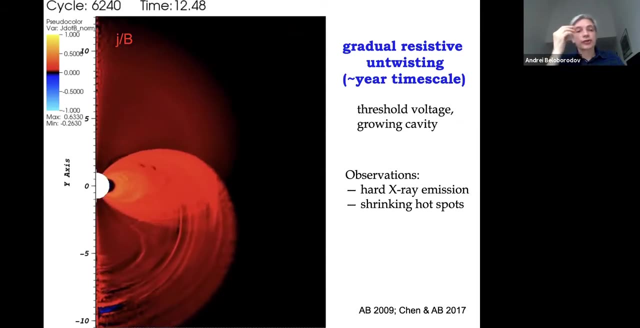 just off the magnetic field. High energy photons cannot be even from magnetic fields. They convert. they convert to curves, So that's how the discharge works. Here is a simulation which shows this discharge. So the simulation is actually symmetric And we simply started to rotate. 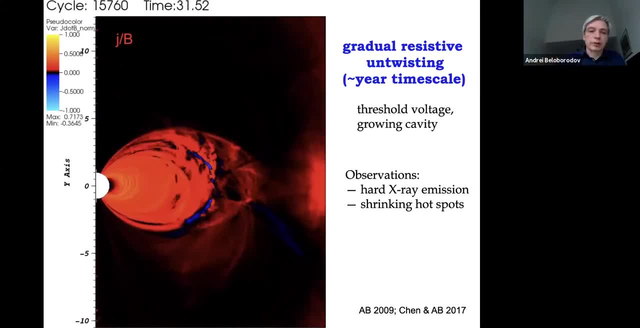 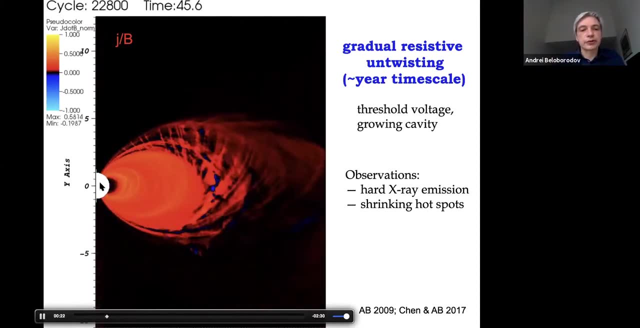 So with the part of the star it should move the big part of the star, the upper hemisphere, Respect to the lower hemisphere, And then you see red is basically the electric current which begins to flow Here. you see this black cavity. 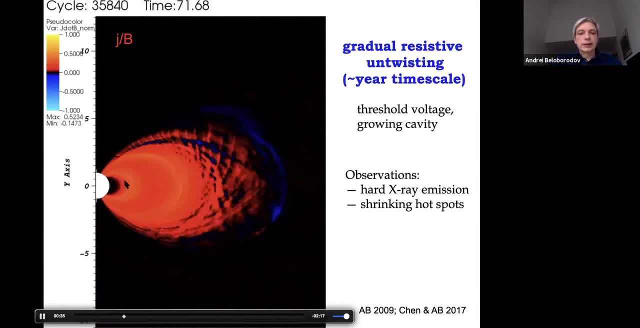 which grows in size. actually it grows very small, So over time and the process lasts. So what we see here in this, by the way, this is a particle itself so-called simulations, And basically we follow individual particles. The model, plasma, is large numbers. 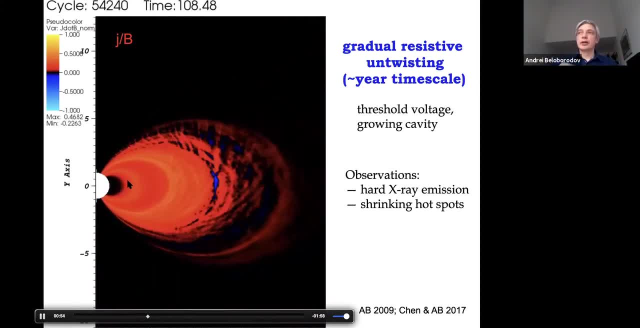 units of digital particles And they move in self-consistent electromagnetic field. So the field leads on a grid. E and B fields lead on a grid And particles are formed individually And the motion determines the electric current that you put in in the Maxwell equations of the source. 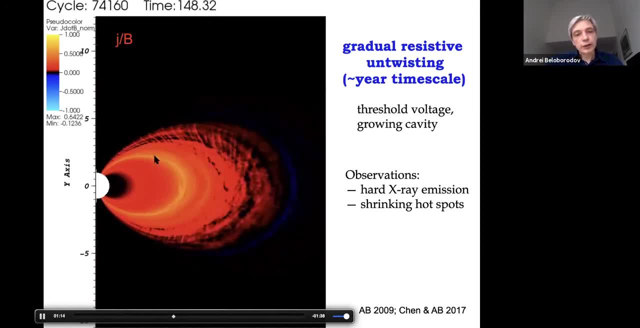 And you can evolve the system self-consistently And with this simulation also implemented this process of electron positron creation. So you see the background for the upscaled right in front of you here And we do see that the system finds a way. 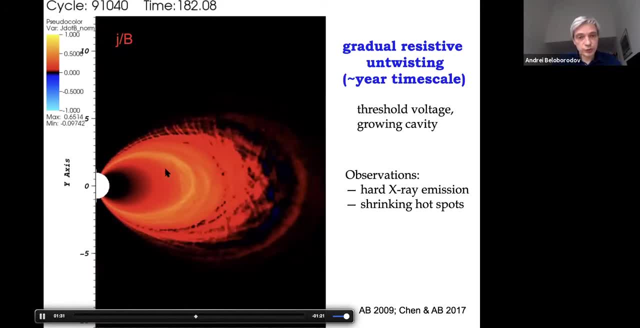 of conducting electric current when the magnetosphere is twisted- And of course this process is deceiving because it requires a final voltage- It can use a threshold voltage to ignite the discharge which is about it's in the GV range, The corresponding time scale- to erase this electric current. 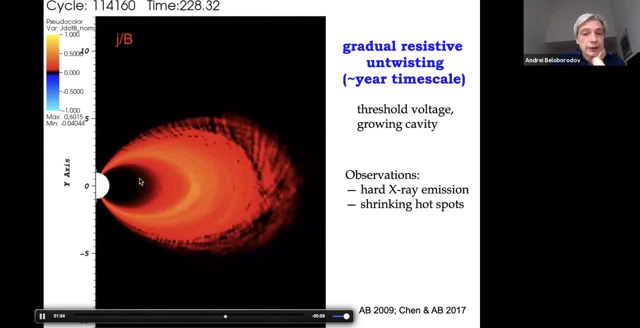 Resistively is like a year. As you can see by now the cavity has expanded. It shows an interesting feature that actually the resistive process works kind of inside out. Basically what's happening? electric currents that used to flow along the magnetic field lines. 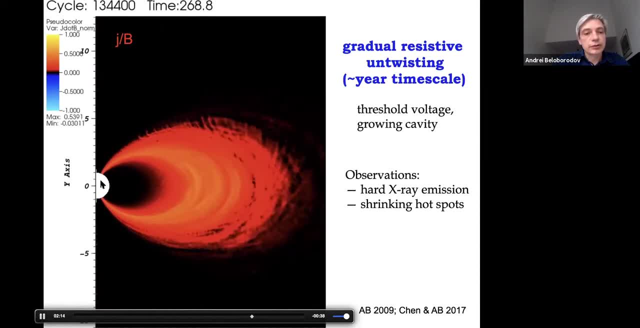 They got erased and they are now closed below the surface. This is ideal conduct to the start. So the currents that flow up there, they're still there. They just close along the surface And then, layer by layer, like onion structure, you remove these currents. 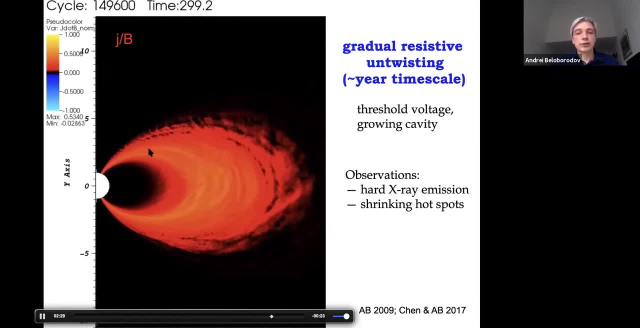 So you launch a front that erases electric current in the magnetosphere on a year time scale. Okay, this is the theoretical picture of magnetospheric activity which results from surface. motions of the magnet are driven by these internal processes and the whole diffusion over it. 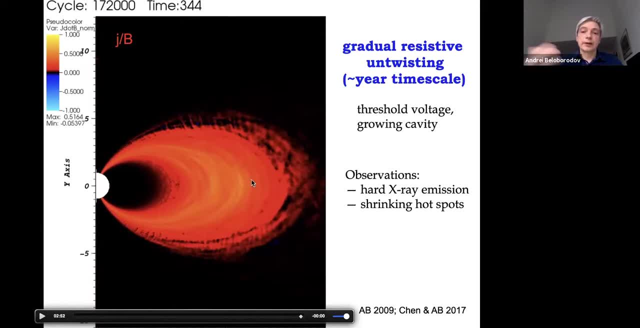 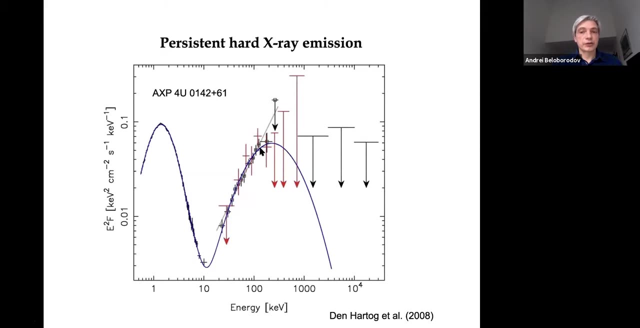 The observational outcome here is that, of course, this region produces no thermal x-rays, hard x-rays And another- and, by the way, this is just an example of a hard x-ray spectrum- the compartmentalizing, the quasi-thermal component. 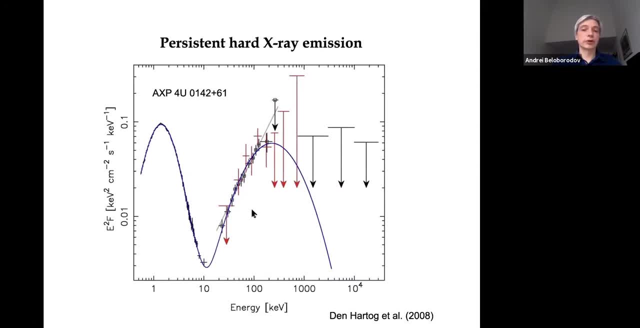 comes from the surface And there is this beautiful, no thermal hard x-ray component. It's quite consistent with this theoretical feature. We see the moment is here. It is Hard x-rays. I showed how this front erases the electric current. 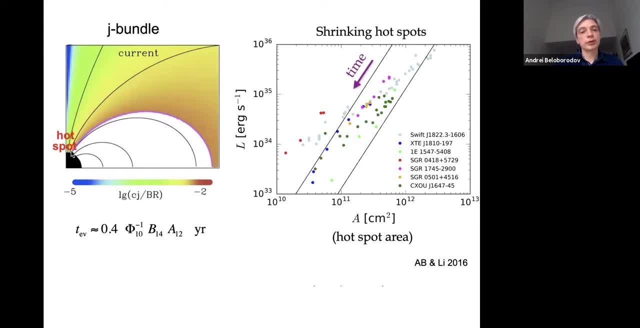 in the magnetosphere and how you can expect a hotspot at the footprint. These particles accelerate in the magnetosphere, then bombard the neutron star and they produce a hotspot. And actually you expect this hotspot to shrink with time as the front progresses right. 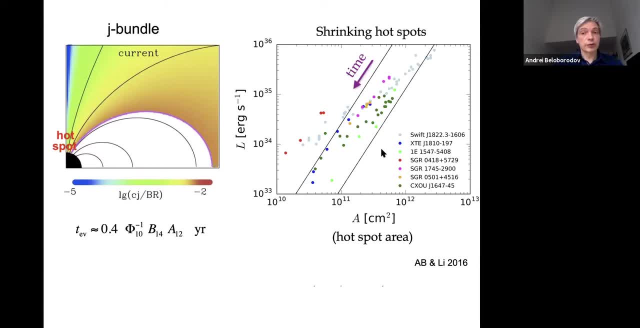 The spot becomes smaller and smaller, And similar hotspots- shrinking hotspots actually- And similar hotspots- shrinking hotspots actually. And similar hotspots- shrinking hotspots actually. So these are several objects where we started to show hotspots. 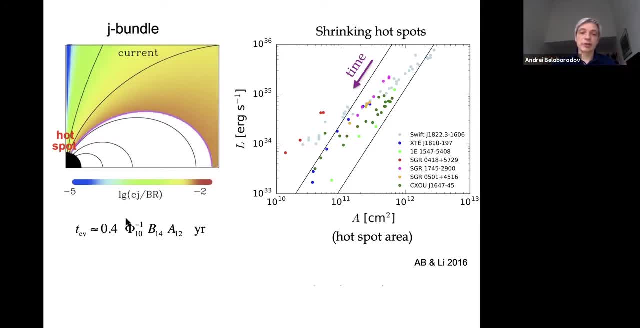 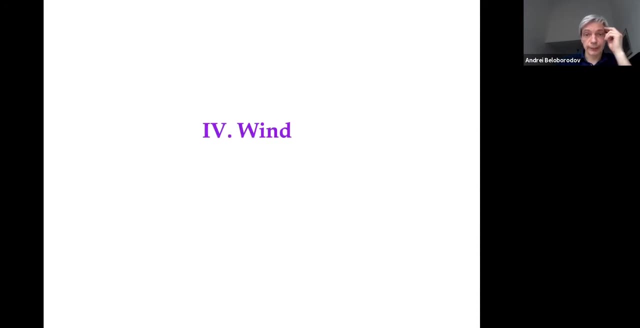 or the trends in the magnetosphere, And then, over time scale, consistent with expectations, months, years. sometimes the hotspots shrink with time, So it looks like we may be observing this process of contrasting. So now let me move to the wind part. 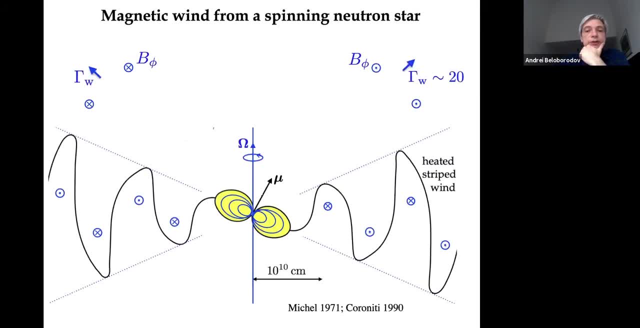 So now let me move to the wind part. So now let me move to the wind part. I'll just comment briefly that any rotating neutron star, magnetized, should be producing the wind. This is the canonical feature of the wind. So omega is the rotation angle of the moisture of the star. 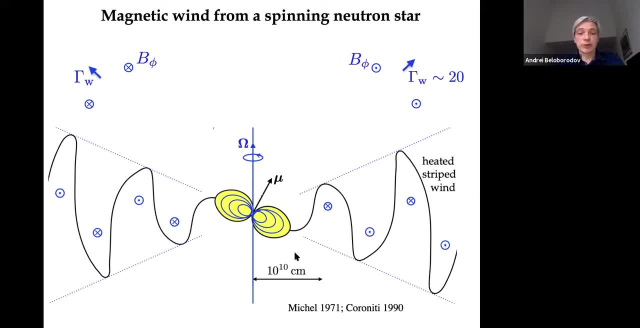 Nu is its type of moment And there is plasma around it And that can force photos and create a new star. And, without going into detail, just let me state here that this is the picture of the wind that you produce outside the lights of the light. 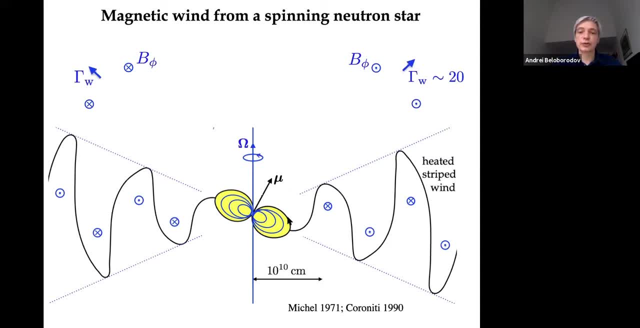 So the light cylinder is the distance from the rotation axis, where the core rotation velocity is equal to the speed of light. So the plasma can rotate this yellow zone with the star inside the light cylinder And it cannot rotate outside the light cylinder. Instead it forms this pointy flux. 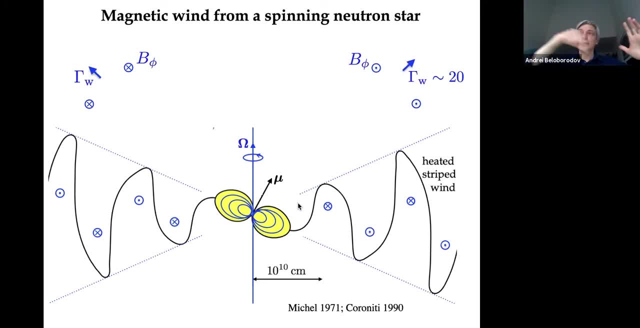 dominated outflow of kind of spiraling magnetic fin lines with alternating polarity, if magnetic moment is inclined with respect to omega. So inside the light cylinder is closed off. Outside the light cylinder there is a wind. This wind is loaded with pure plasma. 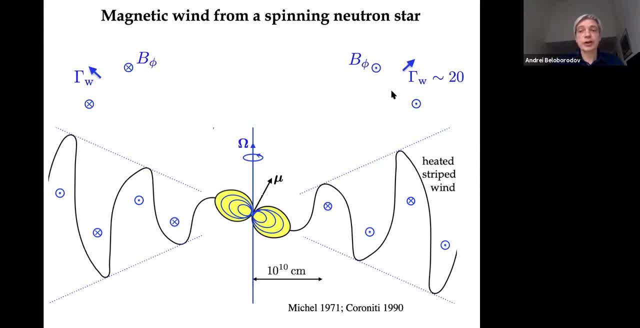 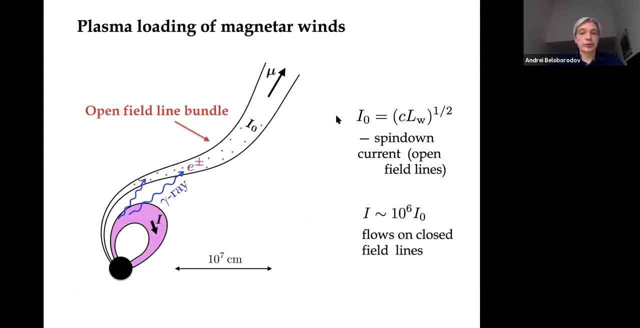 locked in a constant For magnetars? well, it's my estimate, It was not. there's not much work on how fast this wind should be, So here's a slide which shows just one basic point. I think that's the process. 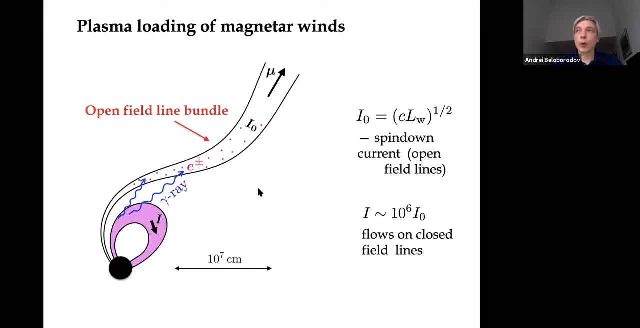 The process of loading of open fin lines that go to the light cylinder and then form this pointy flux. So I note, is the characteristic electric current that all normal pathways have. The magnetic fin lines are twisted at this light cylinder. They form this spiral as you pull up. 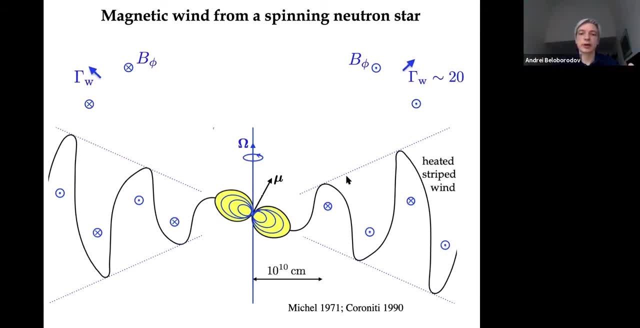 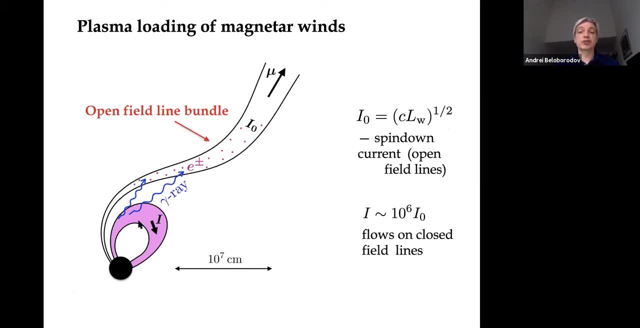 And therefore there is electric currents supported flowing through the light cylinder. This is, I note, Magnetars carry much stronger magnetic currents, million times stronger in the closed zone, simply because they flow in the region of much stronger field, The light cylinder of the magnetars. 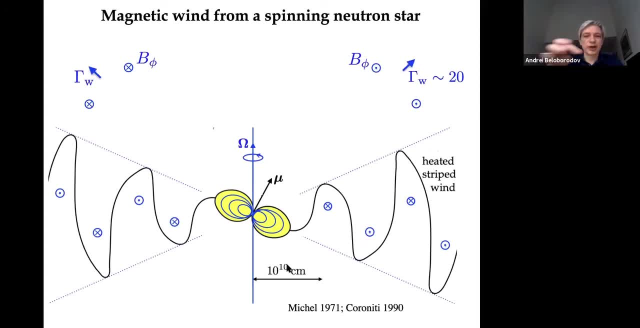 that the radius of 10 to the 10th centimeters, because they're not classical data, so they're all to this one second period And so there's not much magnetic flux actually going through the light cylinders. The light cylinder is five. 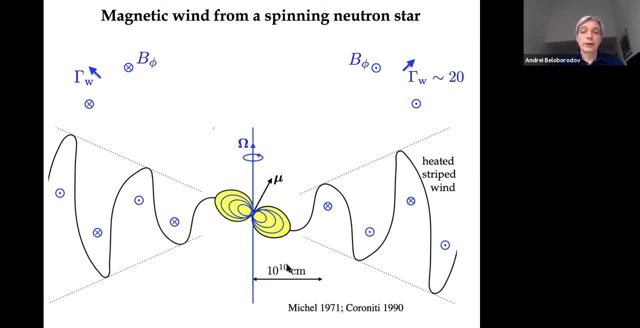 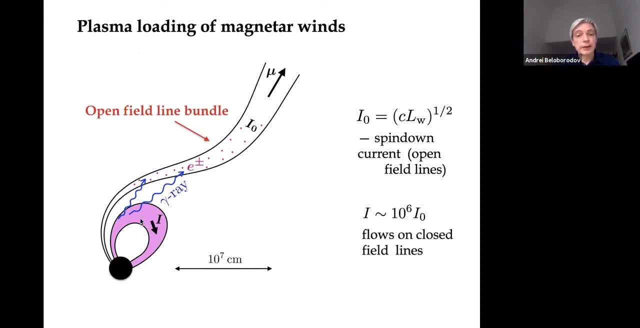 like 10 to the four times the radius of this thing, And this closed magnetosphere with stronger filters, which is strongly twisted, carry much stronger currents, And these currents are supported by electron-poison discharge, which involves this photon production and conversion of photons into pairs. 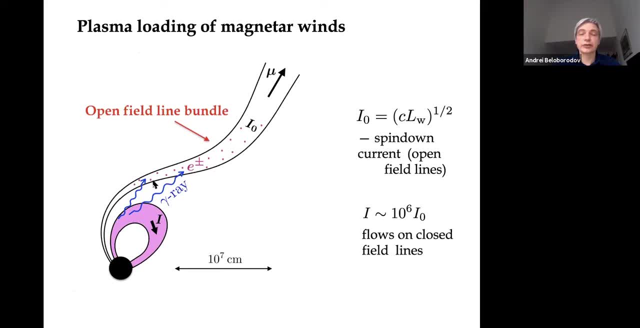 And so some of these photons collide, sorry converges, and then they go away, And then they convert to pairs, also on the open fillets that eventually go to the extent of the light cylinder, And that's how you load plasma into the room. 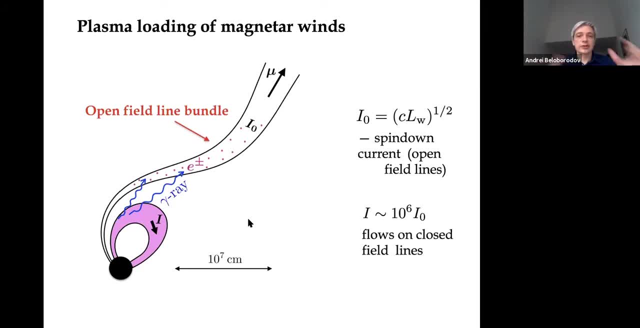 And without giving you further details, it turns out we can estimate the characteristic number of particles that can flow out and it gives you a range factor of the unit that goes out. It's a quarter of 10s. It's pretty fast wind. 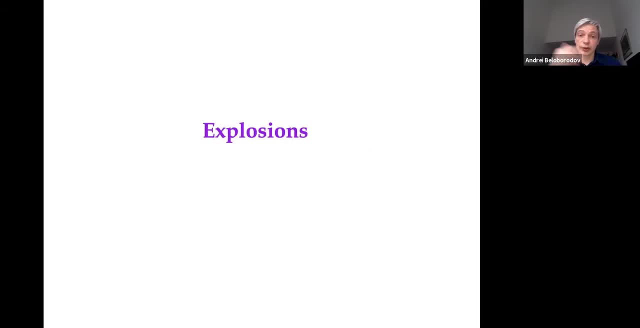 but not as fast as in normal plastics. We have fewer global pair creation rates. All right, So up to now we went through the core dynamics, the crust, the magnetosphere and the wind, And so far the story was relatively sad, I would say. 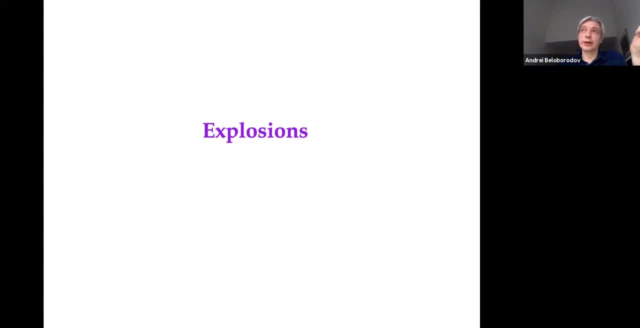 from the point of view of escaping from the magnetic field. but the magnetic field is actually escaping. We're already sampling the flux outside the light. So that's a stunning because the magnetic field is so small with the light cylinder, because the light cylinder is far away from the star. 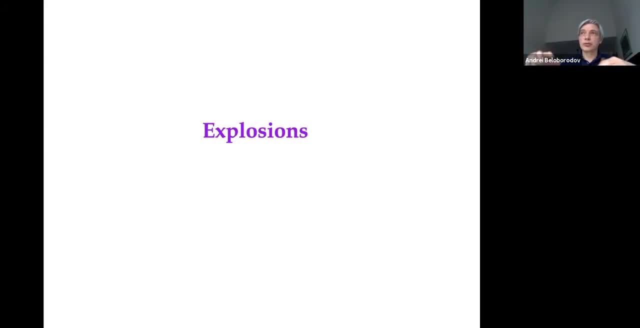 And whatever magnetic field managed to be transported from the core into the magnetosphere, it was erased by the dissipation caused by a combustion discharge. However, there is a process that can finally release magnetic energy into the outer space, and this process is magnetic reconnection. 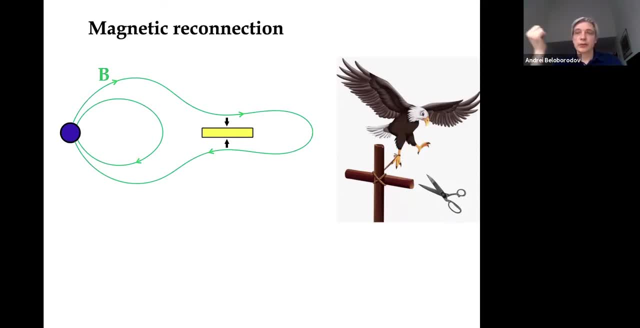 Of course, as long as magnetic field lines are closed and tied to the star, however you approach them, they still remain tied to the star. But magnetic reconnection is precisely the process that produces closed loops that are no longer connected to the star. 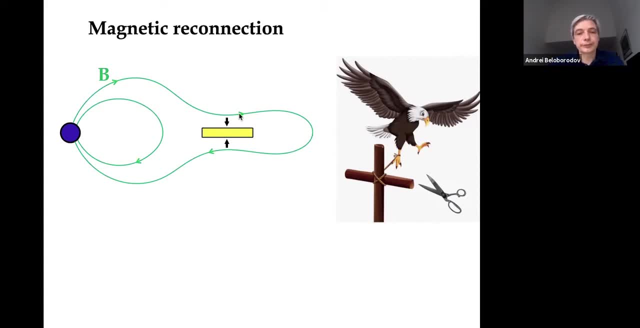 So if you reconnect here, you can delete this magnetic loop. Well, this process is dissipative: magnetic reconnection And here this opposite magnetic fields partially annihilate. so you lose fraction of the energy, but still you can spell significantly magnetic energy as well. 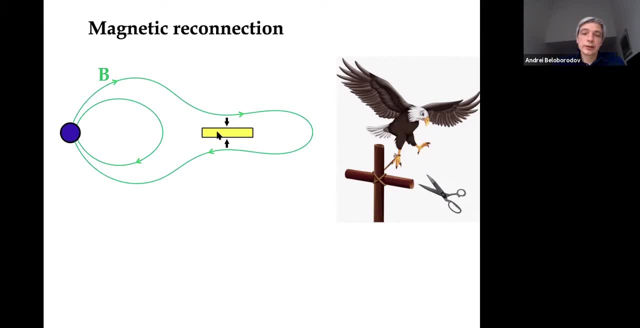 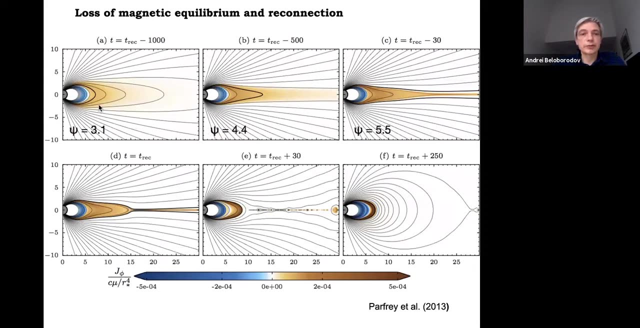 Now there are a couple of ways. I'll show you a couple of simulations how this can happen. This is more, this is a symmetric simulation where, again, you take upper hemisphere of the star, begin to rotate it slowly with respect to lower hemisphere. 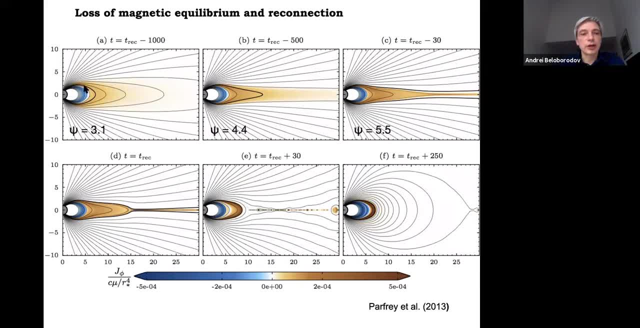 twisting out the magnetic fields attached to the star. One thin line is the color is J5, the little tangents. One thin line is J5, and the other one is highlighted there and it's like a thin flat line. 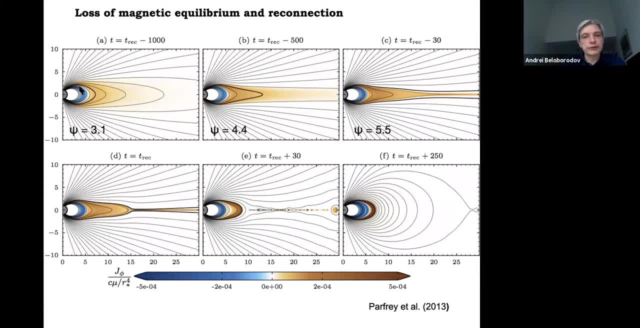 And as you begin to twist strongly with a few fields, the magnification inflates. You can see that this particular thin line becomes more and more extended and eventually it opens up And there is an instability that when you impart magnetic twist in radiance, 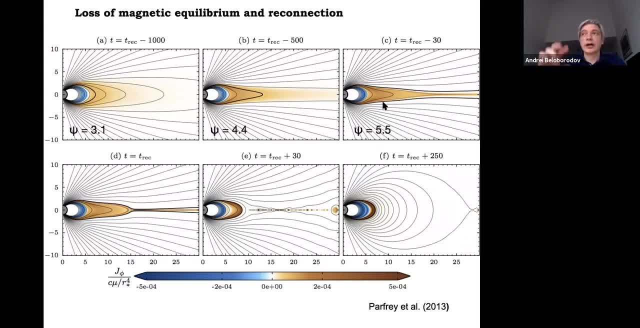 something like four or five. then this configuration becomes unstable. So slowly the field inflates and then boom at some point it becomes unstable from a very thin turn sheets according to opposite magnetic classes, this way, right, Right, And then this turn sheet between them. 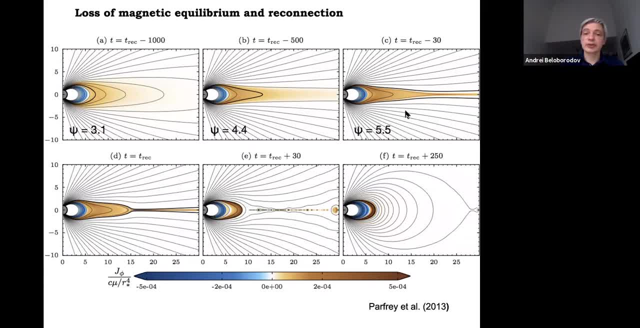 and this fault is known as fault-magnetic collapse, and then becomes unstable to so-called tearing mode, because this turn sheet begins to break up into threads, current threads, And this is the reconnection process. You can see the simulation. So that's one way of doing it. 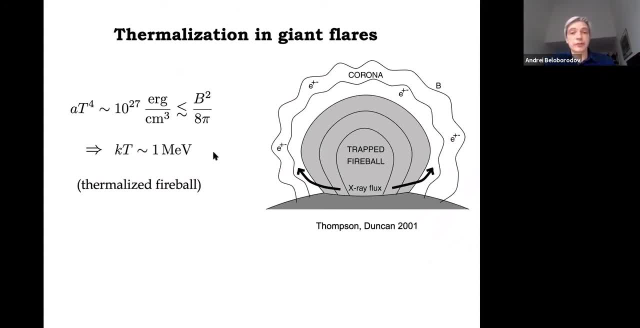 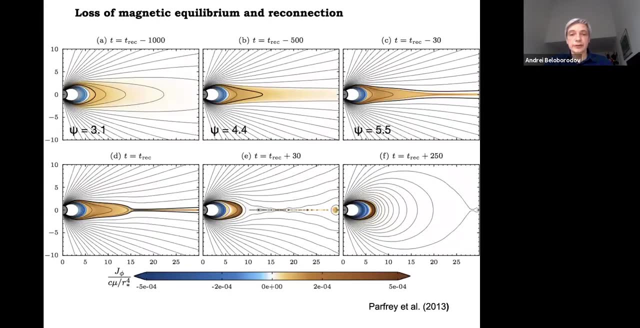 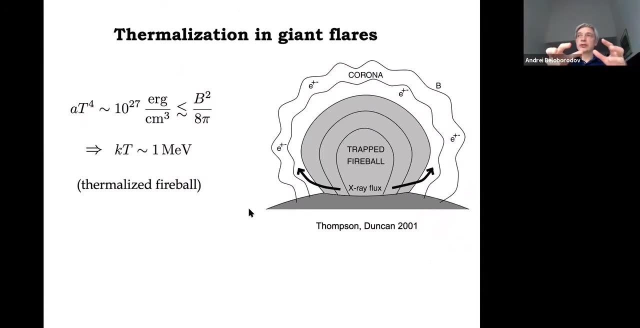 They're very high. This is what we think is happening in giant theories of magnetize, Because this process is dissipative and you will lose a lot of energy if it happens close enough to the star and where you have to store magnetic fields And basically you take a fraction of magnetic energy. 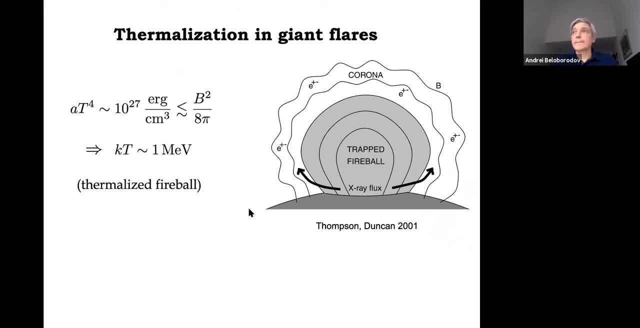 convert it to heat. Suddenly, when the magnetic energy is so high like this- here is 10 to the 14th, 10 to the 15th gas- you can calculate your thermal. basically, you convert it to heat. This energy is completely formalized immediately. 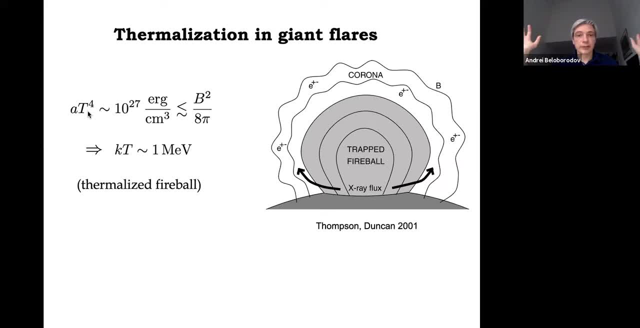 All the rates are huge. So you have so this called full thermodynamic equilibrium. You create electron-phoiston pairs, in particular that correspond to the temperature, and you form an optical thick electron-phoiston fireball trapped in the magnetic, in the magnetosphere of the star. 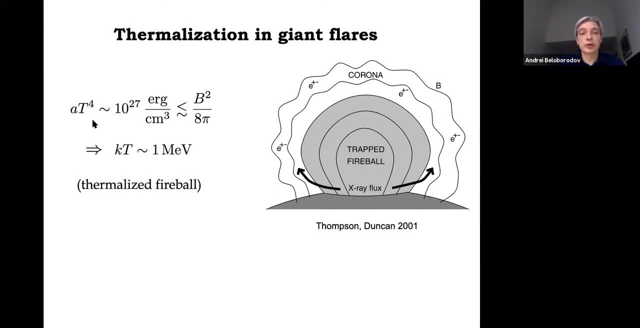 And the typical temperature of this fireball you can estimate simply by creating light-body radiation energy density to a fraction of magnetic energy density and you get temperature called MeV. So that's why we have a lot of electrons and positrons there, because one MeV is above the rest of us. 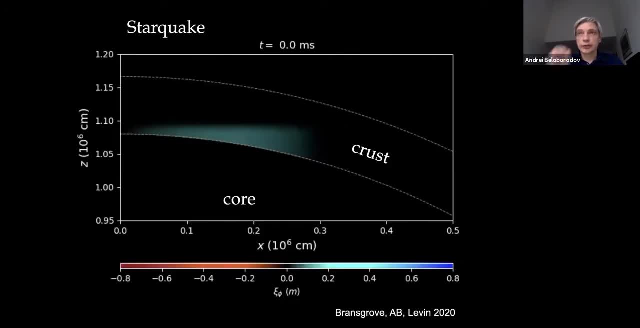 Another way of producing reconnection and releasing magnetic loops from the star is much less energetic When you have a starquake. so what is a starquake? A starquake really? what we mean by starquakes magnetizing particles is also earthquakes. 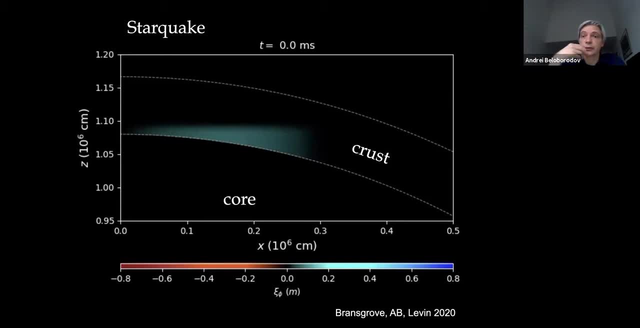 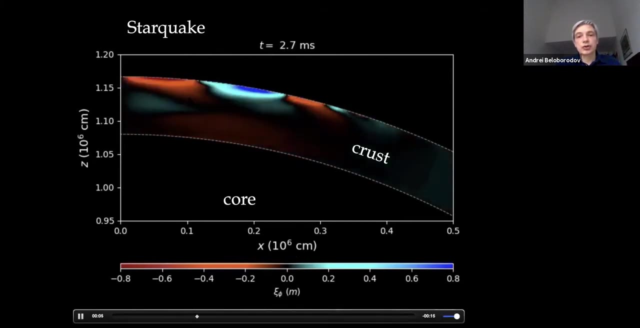 it's similar. So you excite oscillations of the earth. So here you excite shear oscillations of the crust. And these are these. here are just one simulation done by Ashby Gransgrove and our group that shows color, shows the displacement. 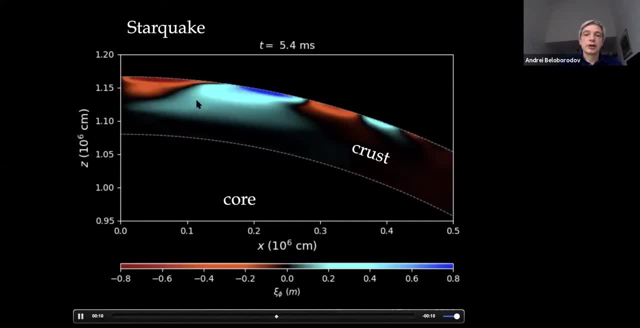 into the plane of the figure And you can see how this shear displacement growth near the surface of the star very similar and the propagated along the surface sideways very much like so called gallery modes with theirdocky modes. 다음에oring的彙果故事. 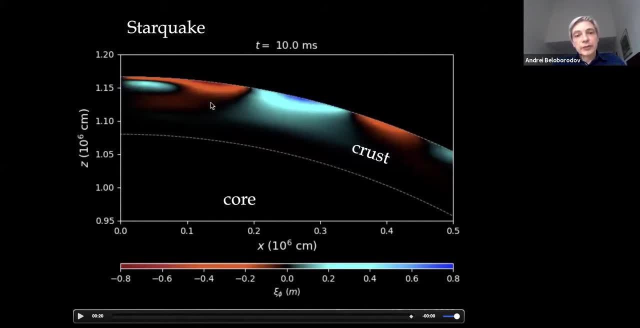 So that's the outward physics here. They have this share oscillations. once we create them, They go to the surface, they go along the surface and they have highest amplitude near the surface of the star. And so the shear oscillations also deform the external magnetic field lines attached to the star. 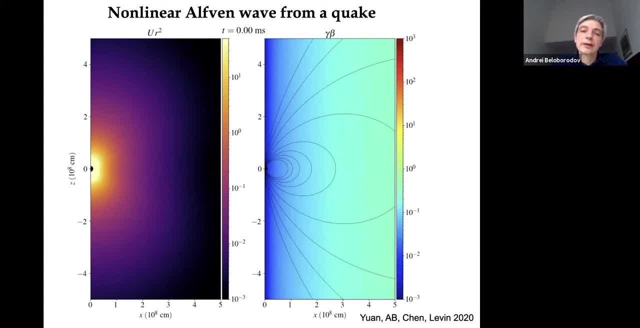 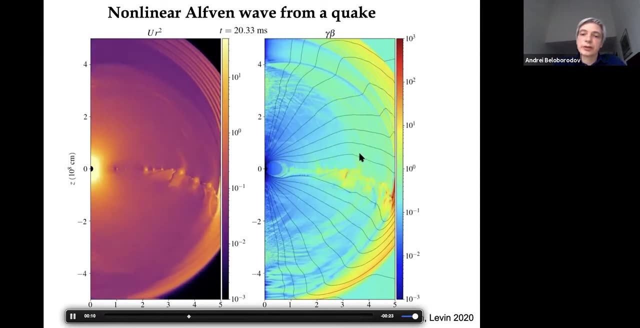 So they launch an alkyl wave into the magnetic sphere And this alkyl wave grows in amplitude because it propagates the magnetic field lines. I'll show you this other simulation. You see black lines, magnetic field lines, And there is a shear alkyl wave that propagates and eventually expels a chunk of magnetic field. 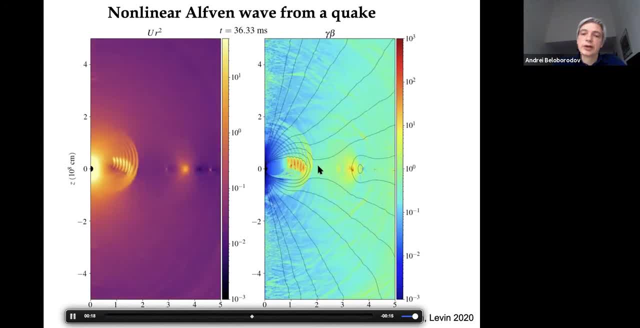 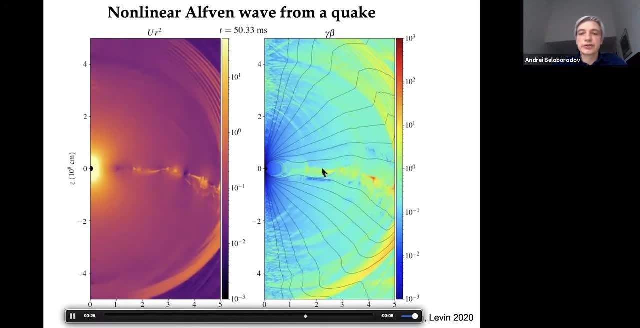 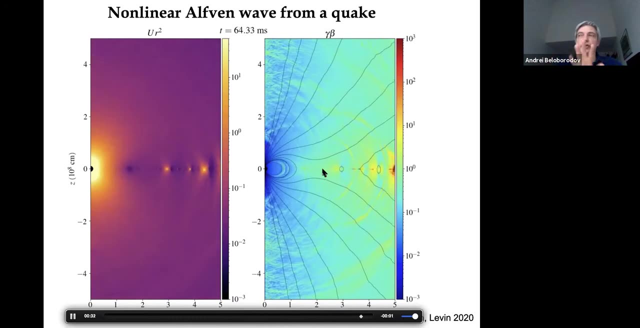 You see a reconnection behind this expulsion event And you see a second alkyl wave. So basically, when you launch an alkyl wave which is initially small near the star, at amplitude maybe 10 to the minus 3, as it goes up into the magnetic sphere along the state of fin lines, 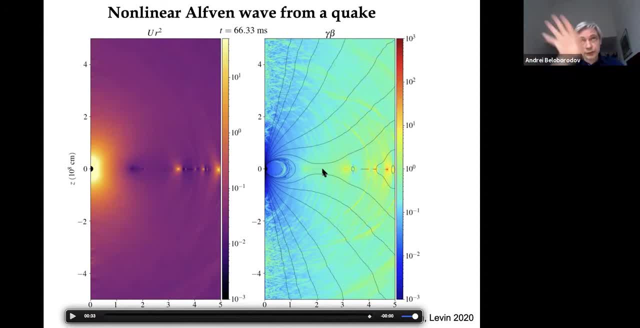 its amplitude grows To conserve the energy flux. the background grows. There's one alkyl for the alkyl field And therefore delta B over B, the relative magnetic energy which it grows, And the wave becomes non-linear. When you launch an alkyl system, it's standard. 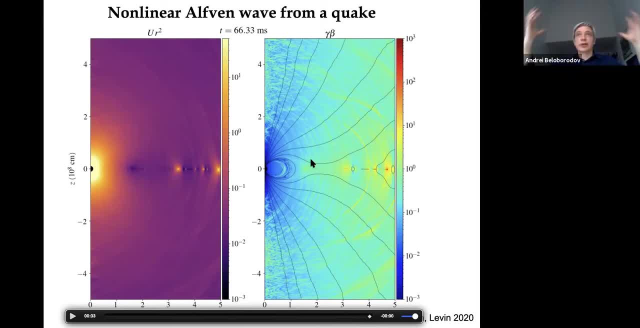 It just says goodbye to the star. essentially, It just feels like: okay, it's on its own. My energy now sees the background energy. I can just keep flying ballistically away from the star, And behind them is the reconnection process. 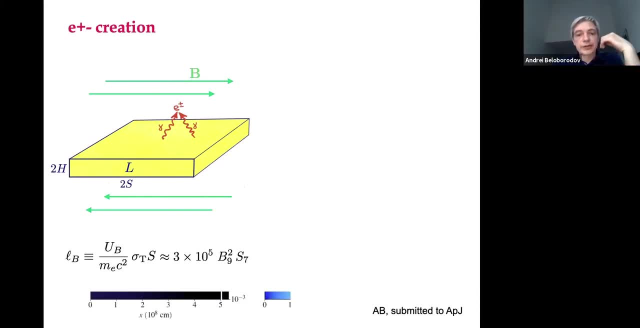 Okay, So this. I would like to say just a couple of words about what kind of emission we may expect from these expulsion events In the outer magnetic sphere, because I think they may actually explain the hard X-ray bursts that we see from our magnetic eyes. 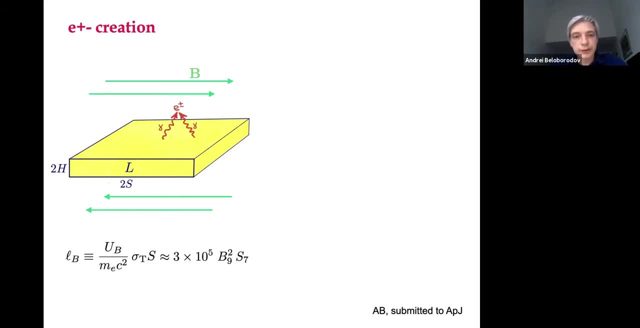 Not the giant waves, but these regular, much more frequent bursts that I showed in the beginning. They typically peak in a dense 50 kV range- the spectrum, the extra spectrum. They last 0.1 second, And so the possible explanation for these bursts. 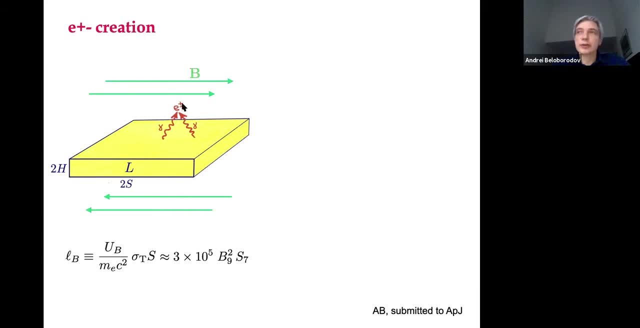 is actually reduced to a clean physics problem. You have magnetic field in a certain size, like 10 to the 7 centimeters, 10 kilometers, or something. 10 to the 8 centimeters, 100 kilometers. Sorry, 100 comes 10 to the. 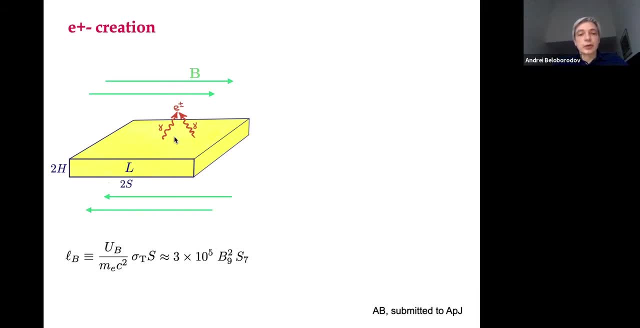 10 to the 8 would be 1000 kilometers, And so you have this characteristic size and you have magnetic energy density. That's all you have in this problem. And imagine now that this reconnection process converts this magnetic energy into heat. 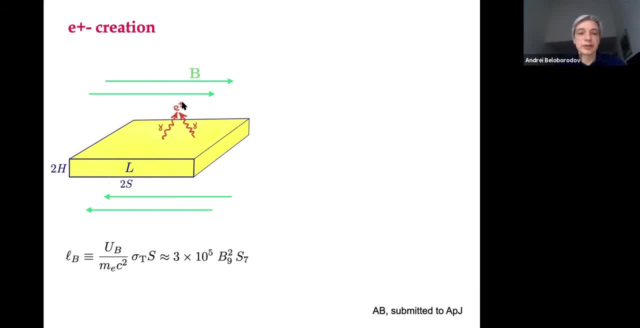 On through a connection. typically it's happening like 10 light crossing timescales of the system. So this problem here is just one dimensionless parameter expressed in terms of magnetic energy, VB and size of the system, similar to this Thomson cross-section. 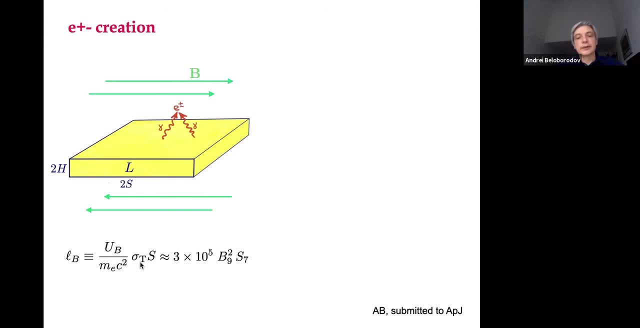 Okay, So you can ask the question in what form energy will come out from this dissipation event. And to solve this problem, you you can. actually, a breakdown is just numerical simulation, So you basically begin to heat particles individually. 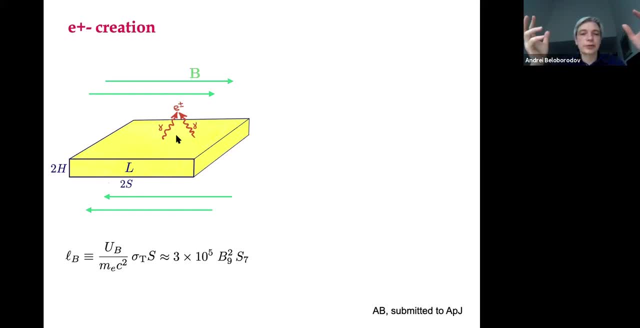 It doesn't matter how many particles you put in the beginning there are a few particles, It's almost like locking. but you put some seed particles there And then you begin to heat them with a given rate, which results from dissipation of magnetic energy. 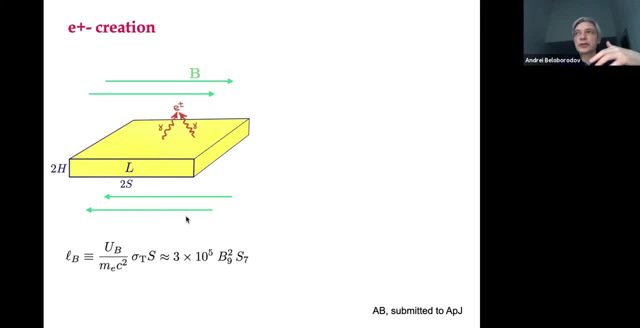 There are some background seed photons and these particles begin to the accelerated particles. heated particles begin to up-scatter photons and generate secondary electron-poison pairs, And you can keep following the evolution of that system. It's basically a radiative transfer problem. 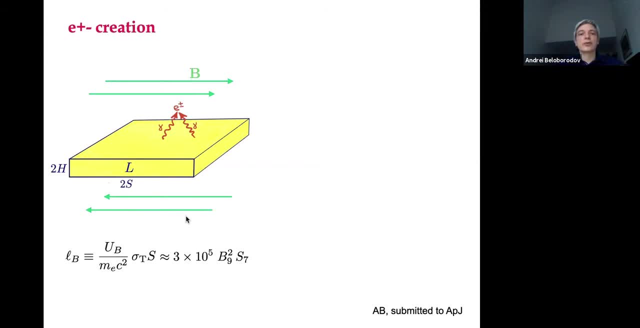 where you supply heat in a certain region and you follow how this heat in the form of photons tries to escape through a plasma which is self-consistently created by photon-photon collisions, turning into electron-poison pairs And, as a result, 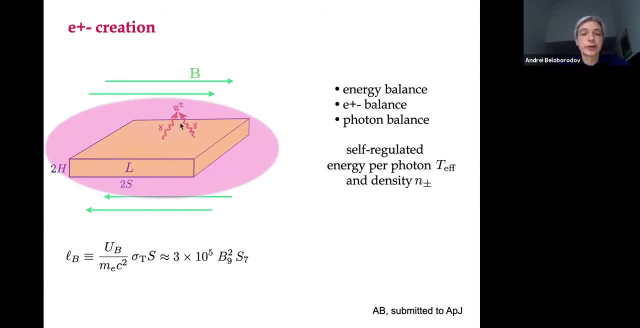 what you find in these simulations is is that this region, heat region, dresses itself into optical thick electron-poison cloud And it self-regulates to sustain about 0.1 electron-base mass per photon because, if you begin to, so basically, the system produces enough photons. 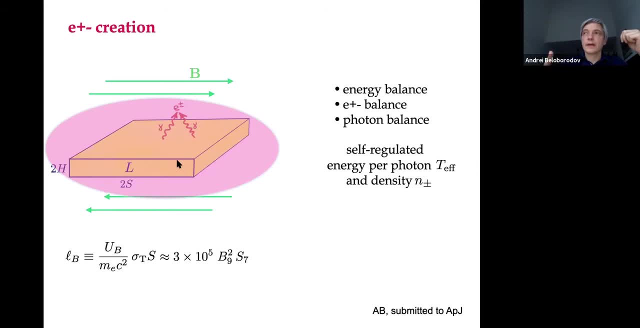 so when they share energy between them, not too many of them are above electron-base mass, unless they start to overproduce the number of pairs and the pairs begin to produce even more photons. and these self-regulations, like feedback loops, make sure that the temperature is not too high. 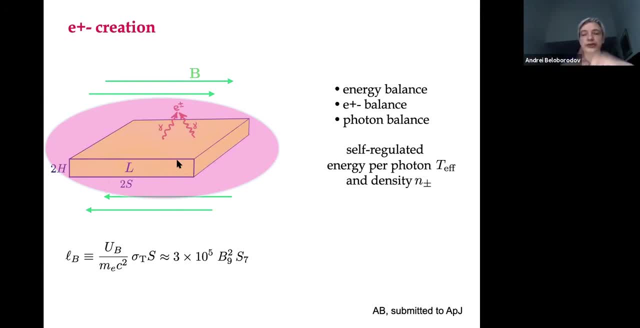 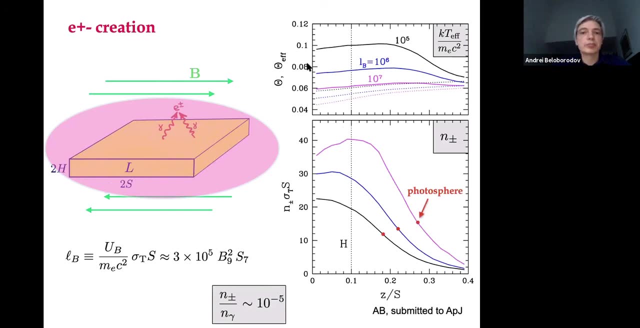 brings temperature back to lower levels. So there is a self-regulation process that controls the temperature in this system. to evaluate about 0.1 electron-base mass, It also controls the number, density of electrons and positrons. tiny number about 10 to the minus five. 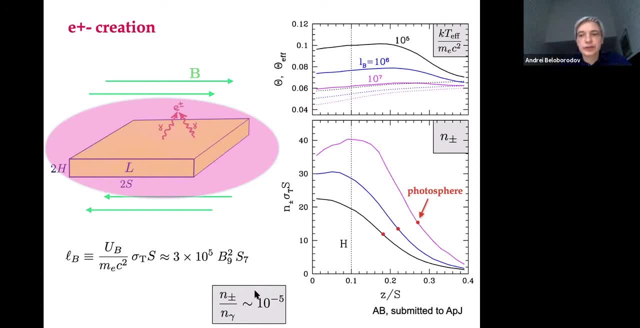 with respect to the photon density that the system generates And you can find from these kind of simulations, you can also find the position of the photosphere, of this cloud from which photons escape freely, And you can find the spectrum that escapes. And here is a theoretical spectrum. 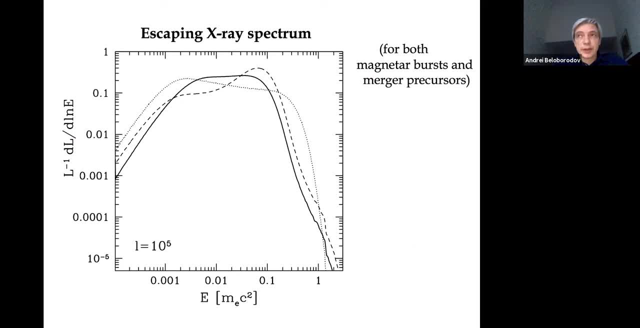 So this is the spectrum that will be emitted by an X-ray burst produced by the reconnection process and ejection of magnetic loop from this star in the outer magnetic sphere, And the burst- the observed X-ray burst- are actually not. I mean, they are similar. 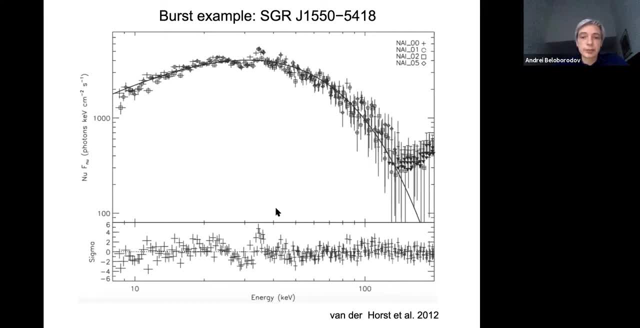 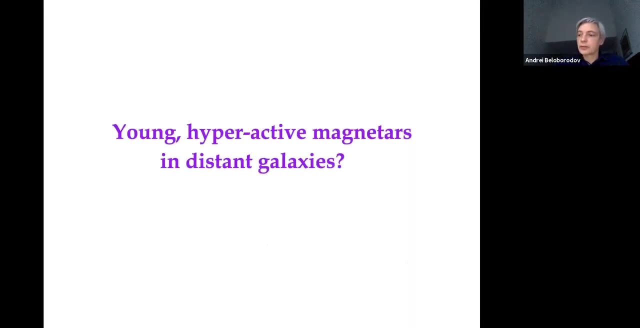 I mean they peak at a similar energy. So you can see here one example: Bursts have a spectrum varying a little bit, but they always peak at hard X-ray bend- a typical moment of that burst. All right, So I have five more minutes, right. 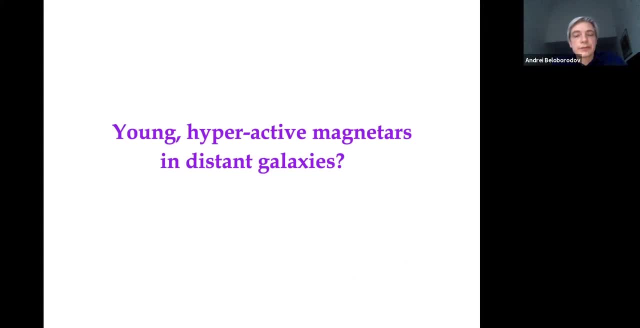 A few minutes, So I'd like to talk briefly about this new emerging connection between magnetars and so-called fast-rated bursts. So the basic idea here is that maybe there are young hyperactive magnetars in distant galaxies which are producing this enigmatic fast. 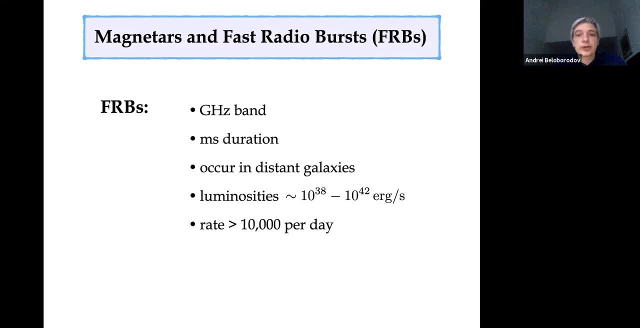 rated burst that we see These fast-rated bursts, gigahertz bursts. they have millisecond duration. They're extremely grand. Their luminosity is up to 10 to the 42 X per second. They occur in distant galaxies. Their rates are more than 10 to the 4. 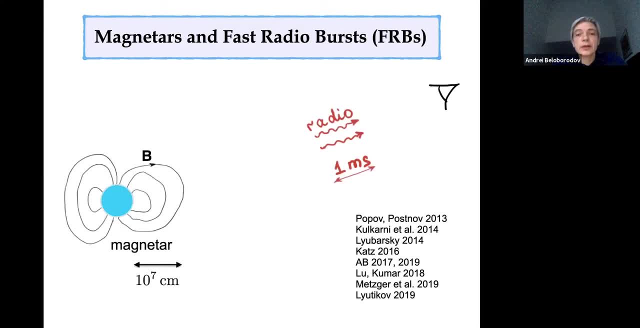 X per day, per entire sky And on thermological grounds. they're discovered only recently. It's a major development in astronomy, particularly radio astronomy. Since discovery of pulsars, They have been associated with magnetars immediately after discovery. so discovery of hyperbeasts. 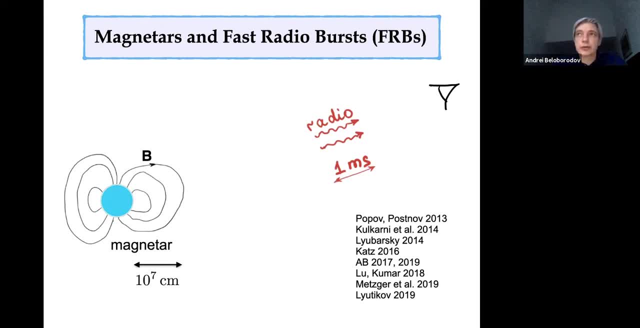 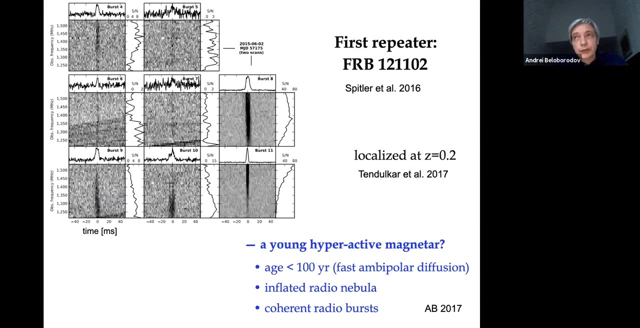 based on the rates and the fact they have maybe second duration. So you begin to think of what kind of source could possibly produce such a burst, And it's got to be a compact object. So the first: many of these bursts are repeating. 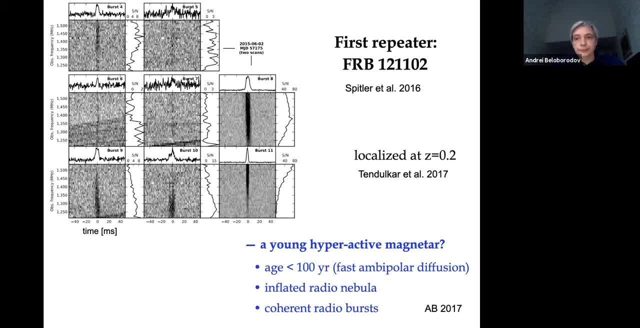 The first repeater was discovered in well. it was localized in 2016 in a distant galaxy, And I think the most plausible explanation for this repeater is the is a young hyperactive magnetar. So basically it all comes to that picture. 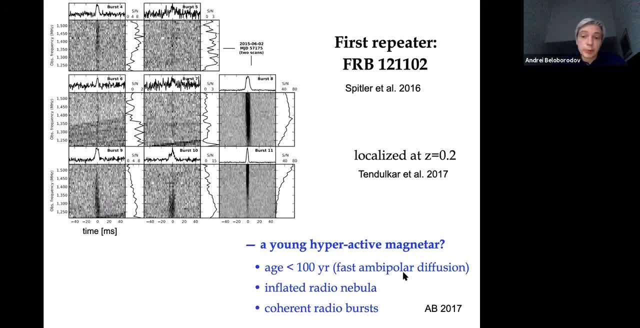 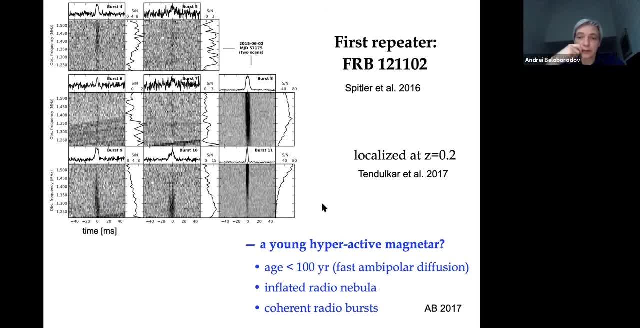 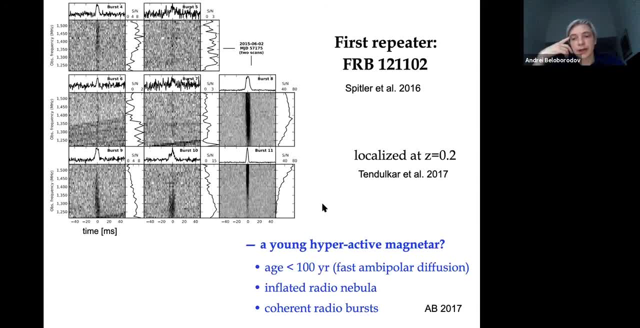 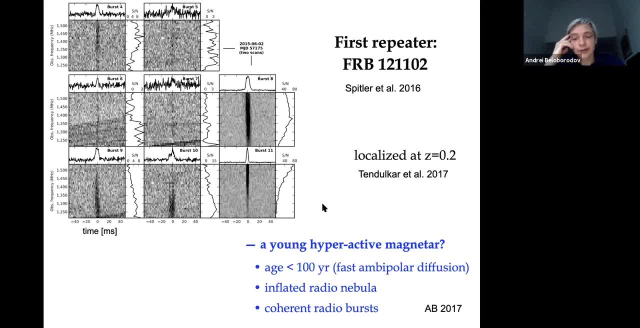 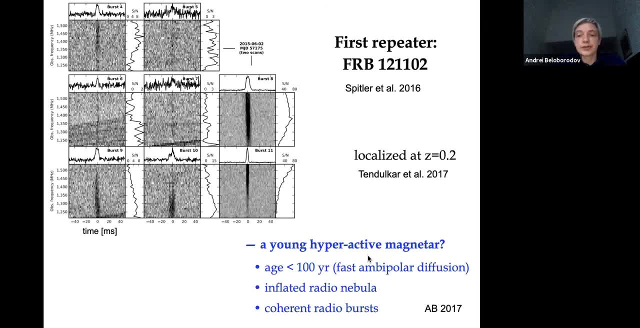 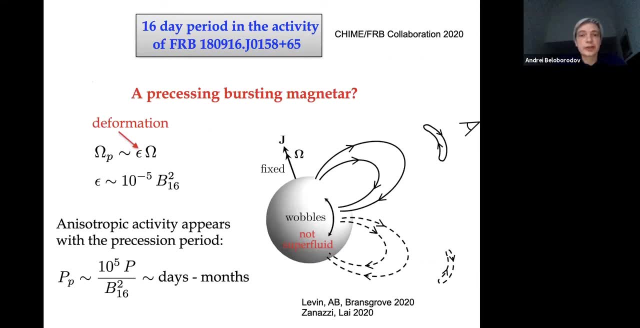 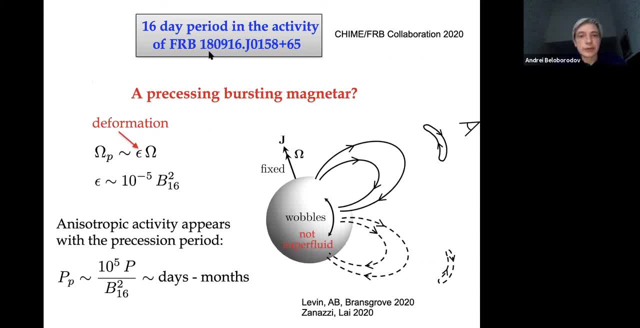 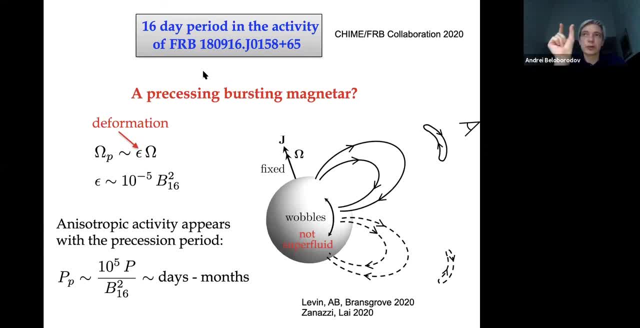 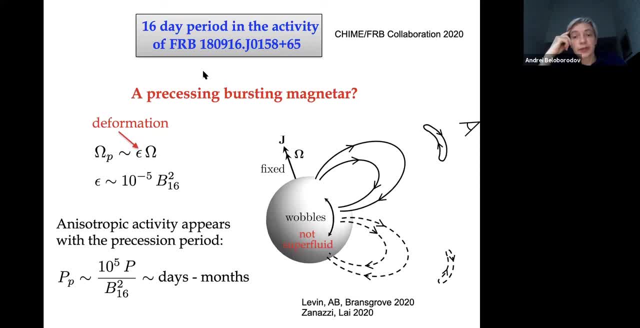 they don't precess because they are most likely superfluid. They are old enough to be cold enough to become, for neutrons to become superfluid. Superfluidity does not allow precession, because what would happen? well, superfluid core. 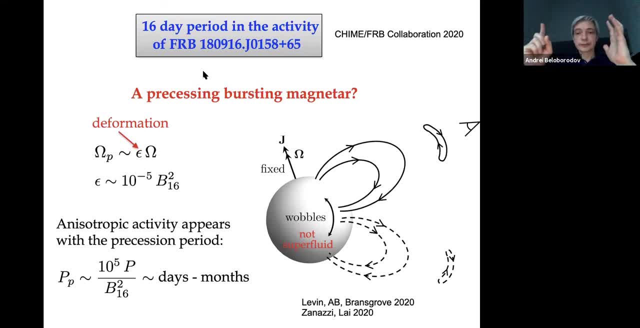 the rotating core, vorticity is quantized, And so you have this array of vortices. If the star tries to precess around the angular momentum, you're basically trying to push the crust, and with the magnetic field which would have to cut through the vortex lines, 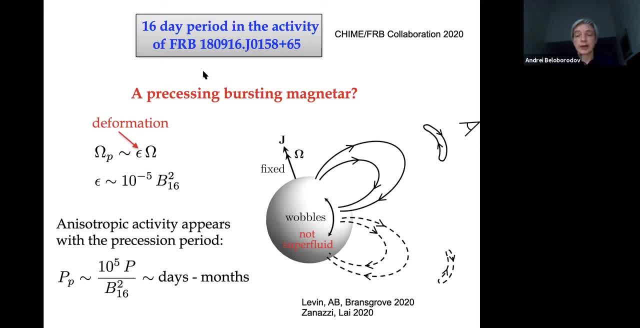 It's most likely the dissipated process not really allowed. However, if your star is not superfluid, that is, it is superfluid if it's hot enough, that is, the magnetar is hot enough to be not superfluid. 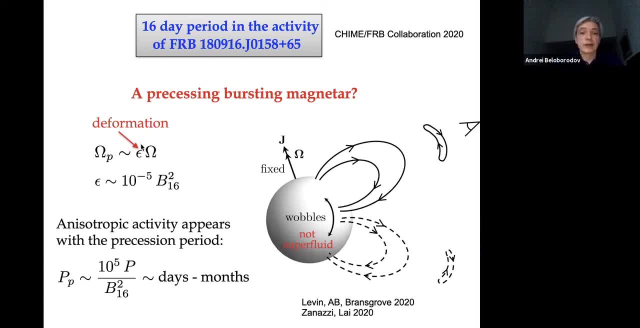 then it can actually expect precession. This precession period is determined by how strongly the star is deformed And it is deformed by Hooke stresses of the magnetic field and field of 10 to the 16 gallons expecting magnetar is deformed at this level. 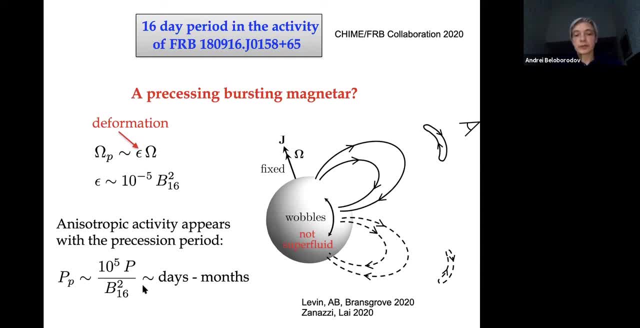 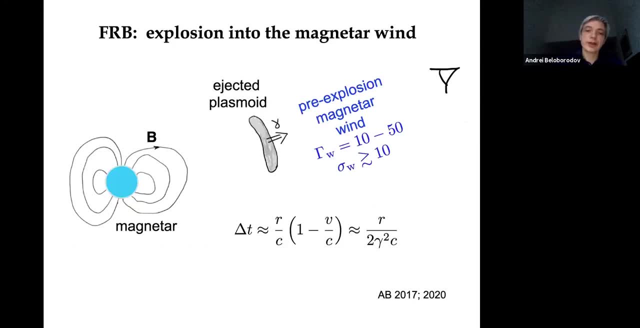 10 to the minus five, And then you get the period of precession of about days to months, which is consistent with the observed precession period. And finally, the last thing is that there's a natural mechanism that should be working in this hyperactive magnetar, producing fast radio burst. 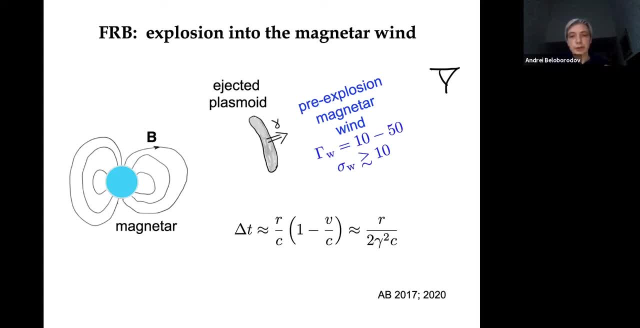 This bright radio emission must be produced by a coherent emission process, And this emission process actually does exist in the blast wave, which is produced by a magnetic explosion driven by this plasmoid, this magnetic loop that was ejected, that I talked before about, right. 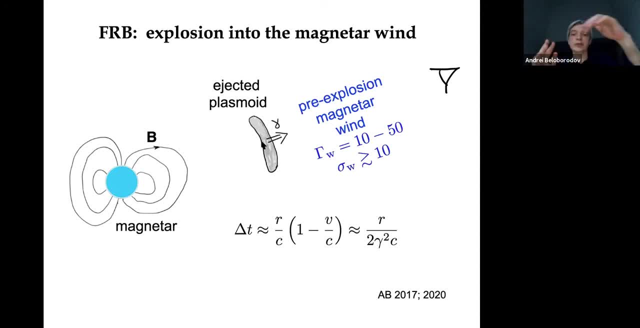 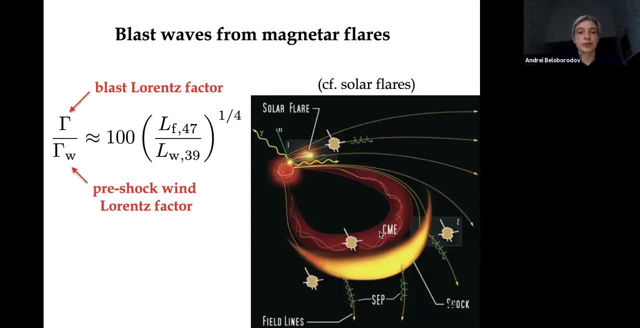 So this ejected magnetic loop, it drives, it accelerates to very high range spots. it drives the explosion, like solar flares drive explosions in solar wind. The only difference from solar flares here is that the whole thing is ultra-lutefacistic. 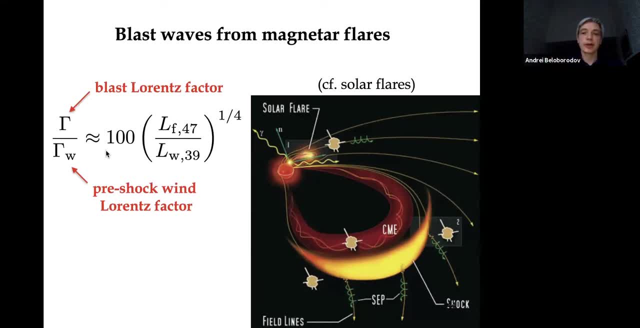 The pre-explosion wind is ultra-lutefacistic and the blast wave driven by this ejected plasmoid is ultra-lutefacistic. The characteristic Lorentz factor is like thousands for the blast wave, which allows, of course, the emission. 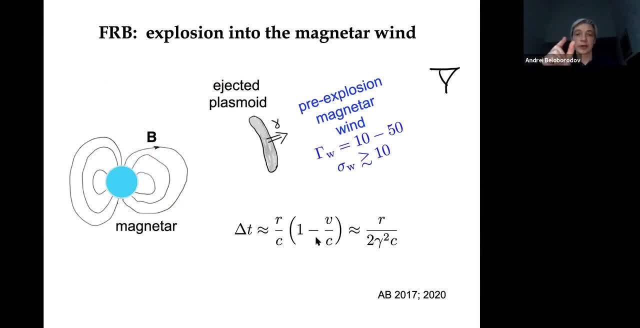 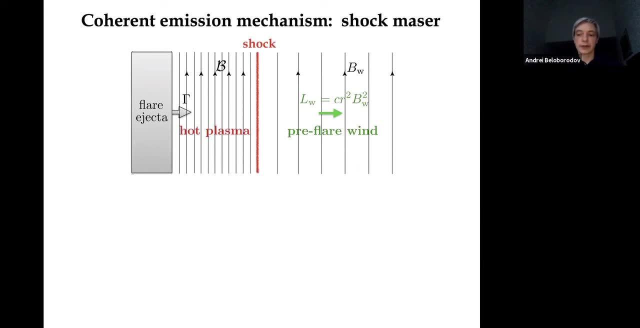 to be Doppler compressed in time, and that's why we observed one millisecond duration. Okay, so the coherent mechanism. that, basically my last slide, I think- is the well. it just illustrates how this coherent radio emission is produced When you have a shock in magnetized medium. 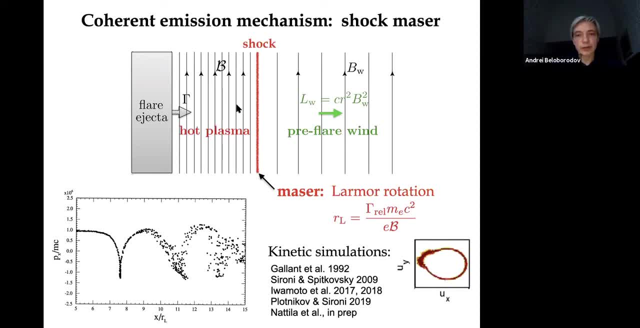 particles crossing the shock begin to generate in the post-shock field and they form a ring in momentum space. So they form a kind of major structure. you see inversion here, right. So a lot of particles in higher levels And this ring is unstable to bunching. 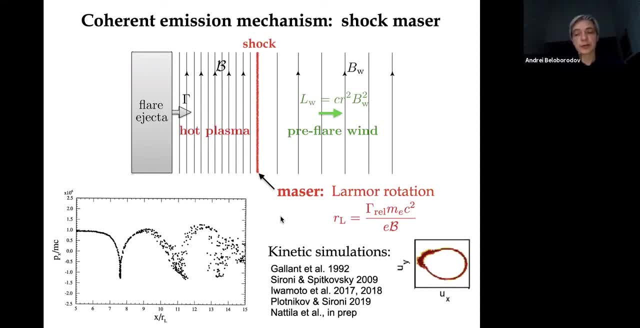 and, as a result, you produce coherent radio emission with frequency which is scales with simple gyro- frequency of this ring, frequency of gyration in the post-shock medium- And there are plenty of simulations. by now We are working with detailed simulations also. 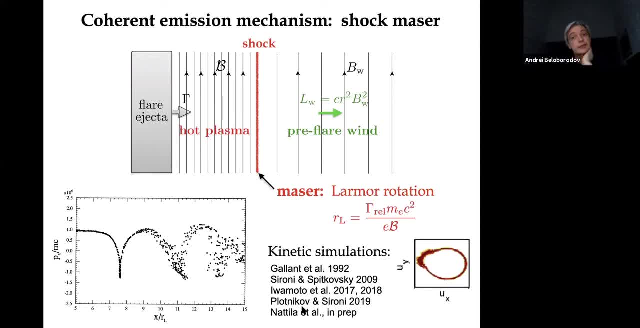 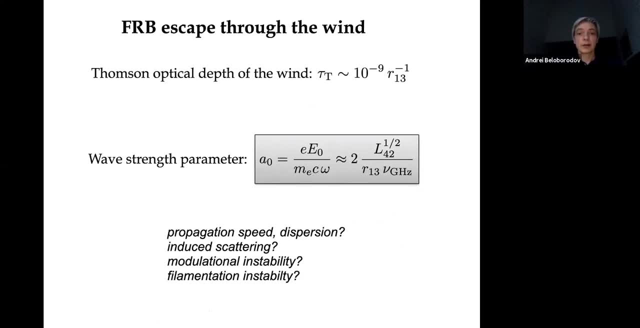 that show elaborated details of the properties of this wind, like magnetic efficiency, polarization, et cetera. All right, skip this. These FRBs they have very strong. they produce electromagnetic waves. Their strength parameters can be way above unity. 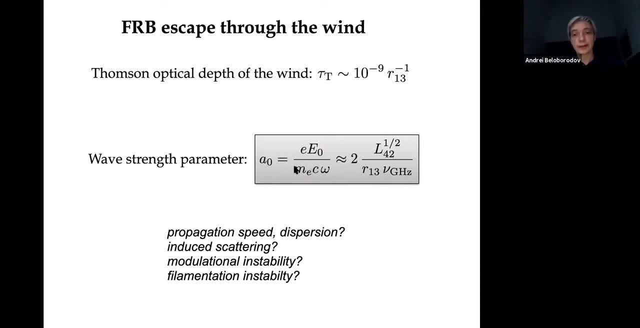 This is what people play with with lasers now. So there is a lot of parallel physics here and questions which are not answered for FRBs here, like modulation and stability, connotation and stability, how this ultra-strong wave tries to propagate through the plasma, the wind as it tries to escape. 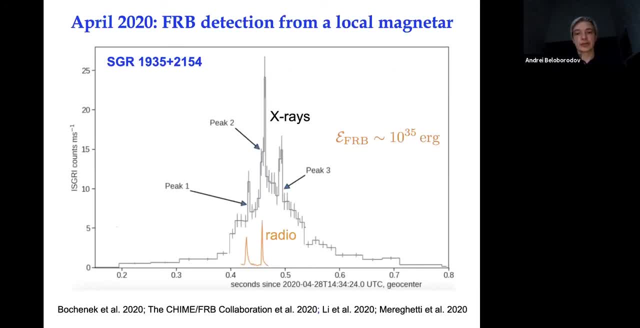 And finally, this is just to give you an exciting observational result which came out a little less than one year ago. This is the first detection of an FRB from a local magnet, So before 2020, April. it was all speculative. 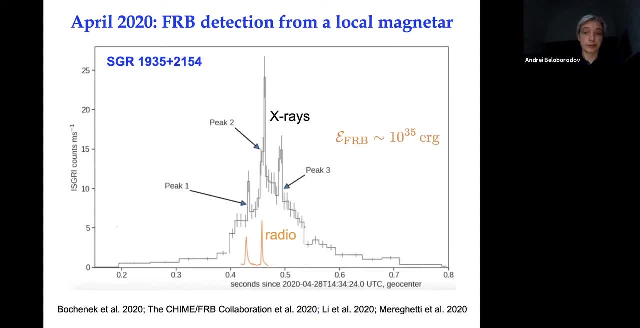 the idea that magnetized produced FRBs, but now we know that actually they do. So one of the FRBs was detected. It was a relatively weak burst, but still it had millisecond duration. It coincided with an X-ray burst. 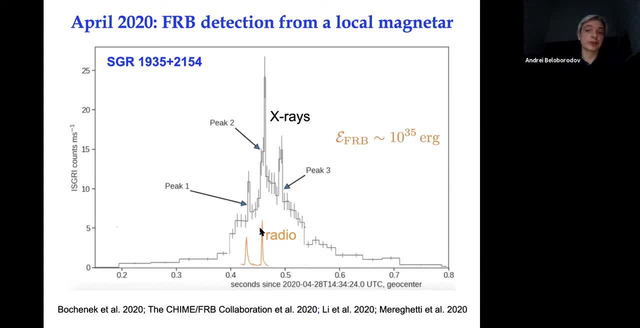 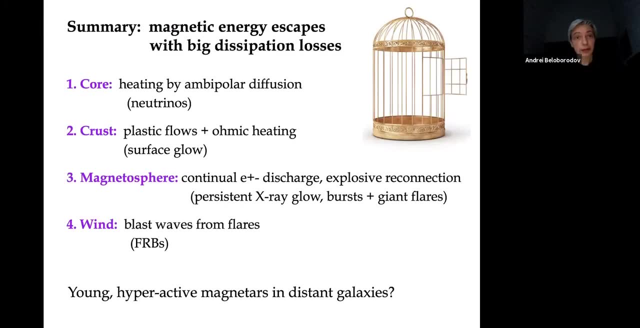 And it, except for its brightness, it looks like normal mass gradient burst. So here's my summary. So, basically, magnetic energy does succeed to escape over time from the star, but it's doing that with big dissipation losses. Okay, Starting from the core, that the first process. 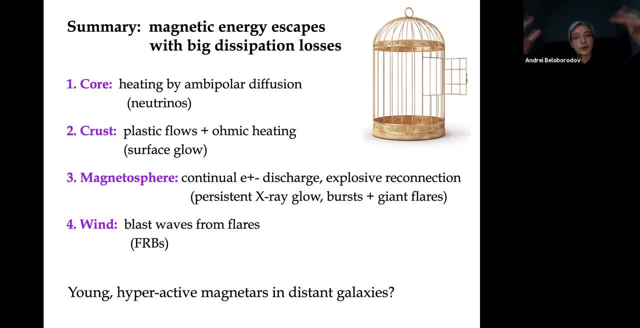 that allows the field, life to move, magnetic field to move out from the star, from the pole, to the fusion. most of it is wasted. It's wasted into neutrino emission. We are fortunate that there are these dissipation processes because this quest of the magnetic energy 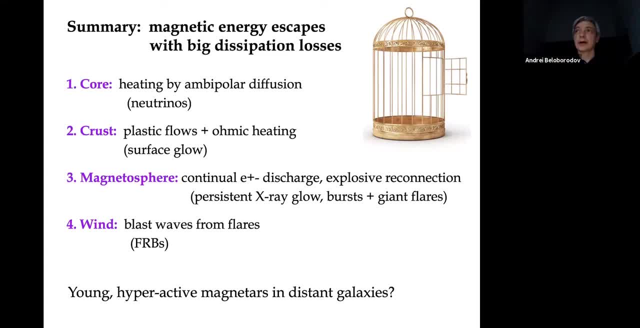 to get out from the star. if it does so easily, it would be completely silent for us. but precisely because it goes with dissipation, that's why we observe this object as bright bursting sources, hot stars like Ambipolar Diffusion Heating. 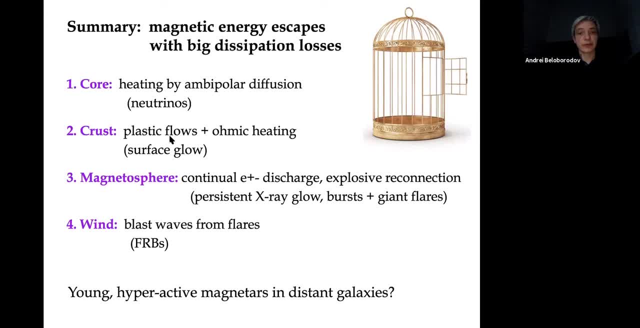 and so on. So we observe the magnetic heat dissipation in the core and mechanical dissipation for plastic flow in the crust, plus possible heat in the crust. They make the surface of the star hotter than it would normally be. There are also particle magnetospheric dissipation. 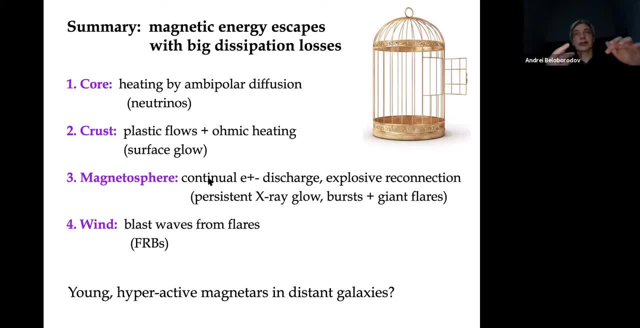 which occurs through, because the magnetic helicity gets out of the star. it generates electron-phosphorus discharge in the twisted magnetosphere. These particles accelerate in the magnetosphere, bombard the star, create hotspots and we observe them And also. 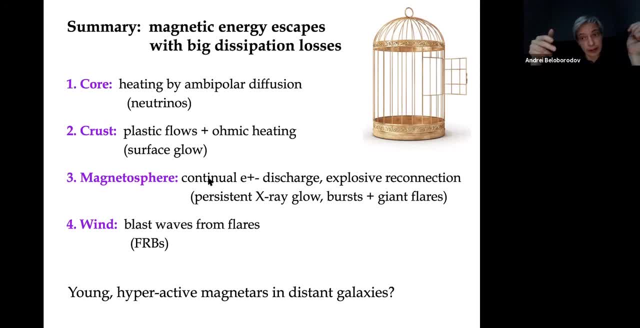 when we over-twist the magnetosphere. finally, the magnetic chunks of magnetic energy have a chance to escape through explosive reconnection. A large part of it just moves out freely, expands from the star, but part of it is dissipated. and that's precisely the dissipated part. 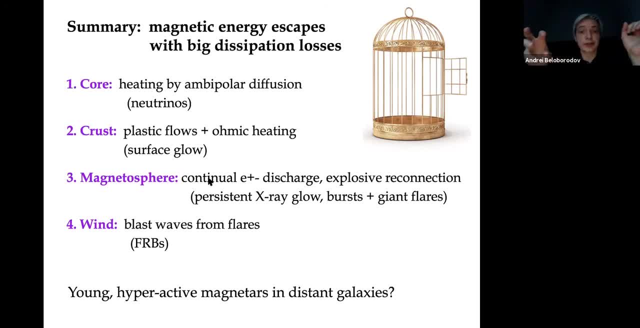 that we see as bursts or giant flares in some cases. And finally, these explosions also launch blast waves into winds of the stars, of the magnetars, And these blast waves naturally have a coherent radio emission mechanism which produce which is so bright, so much easier to observe. 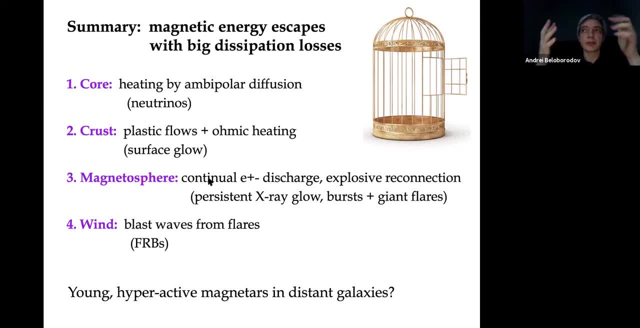 from the radio band, The detectors. radio detectors are so much more sensitive than even optical radiation X-rays detectors, So radio telescopes can pick up weak radio signals easily from very large distant distances, from distant galaxies, And actually this coherent radio emission. 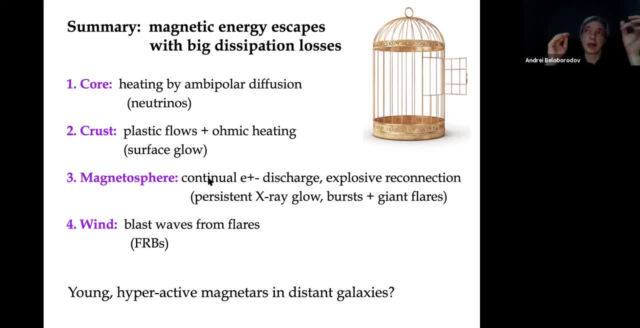 from blast waves from these players are expected to be really bright and easily detectable, And so that may be why we are observing these fast radio bursts, simply because there is a population of magnetars that keep producing blast waves and we easily pick up them in radio. 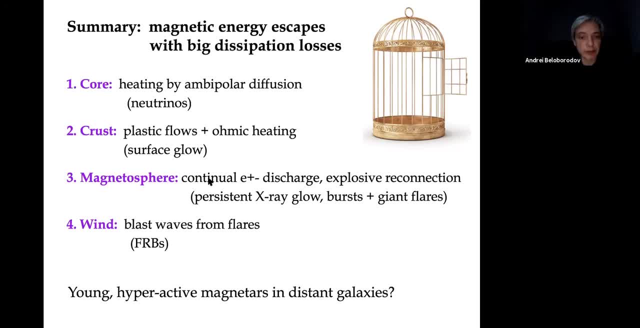 Not so easily in X-rays, not even gamma rays, but in radio, yes, And so I was arguing that these distant galaxies may have many non-hyperactive magnetars which we are missing in the Milky Way. just statistically, we don't see a recently born magnetar. 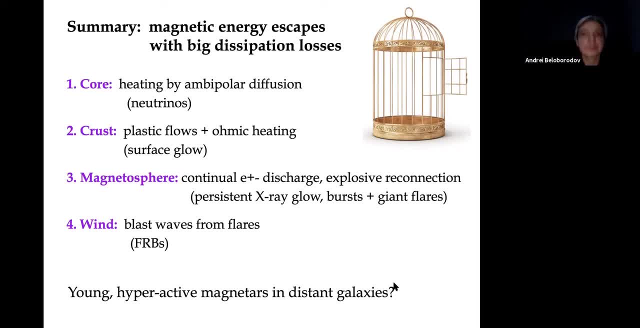 but they can exist in distant galaxies and produce- And I'll stop at this point, thank you. Well, thank you very much for a very nice presentation. We have some questions from the audience, So let's start with Efrain Farah. 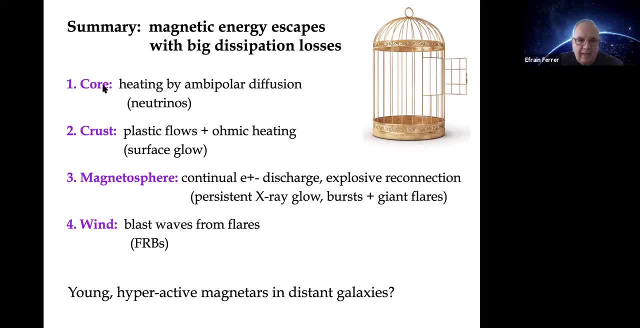 Yes, thank you. Thank you for the interesting talk. I would like you to comment about the possibility to have magnetars with a strange matter, and also to talk a little more about how to get the stability of the field, of the high field that you can have in the core. I cannot tell you much about it. I mean, it's possible, There are works, of course on the transition, but you're going to have strange matter in the core. Things might depend, but I don't know what should happen then. 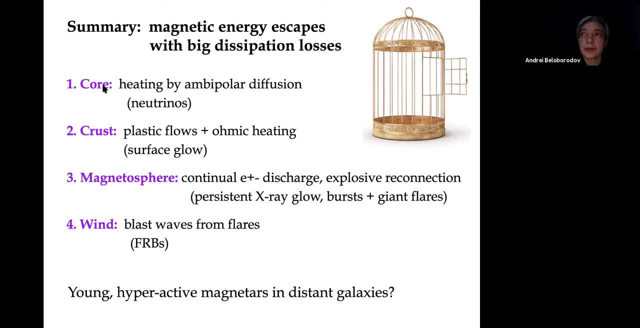 with the magnetic field. I don't think I'm in a position to make any predictions there. The only thing I can say is that the law should depend on the mass, because the higher density this may be, this kind of position may depend. 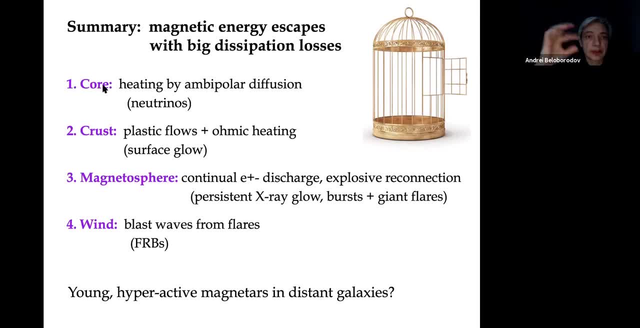 on how massive the star is. Well, you can imagine different classes of magnetars. If you create a really massive magnetar, let's say two solar masses or more, then it will be the most compact magnetar with very high central density. 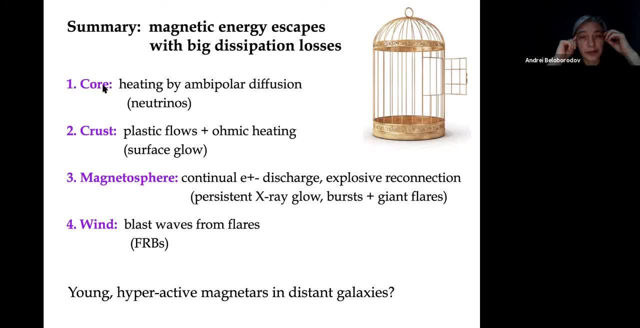 And then you can expect things more likely. There could be a transition there. So it would be interesting. It's possible that there are two types of magnetars, let's say You see what I mean. I mean depending on their mass. 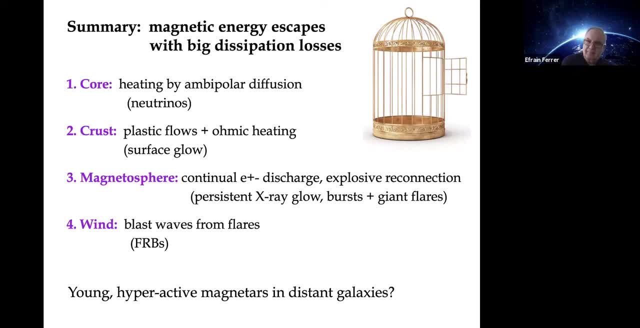 Yeah, another difference Depending on their mass. Yeah, another difference is that if the star is massive enough, so the density reaches 10 to the 15th grams per centimeter, cube seeds in then another qualitative difference that happens there. 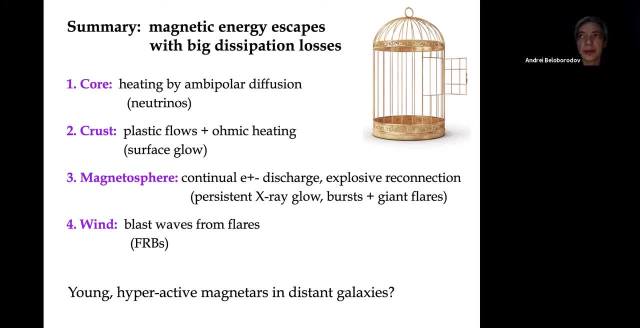 important for this dynamics that I described is that you begin, you activate direct OCA process, which is much stronger neutrino cooling channel, And so, basically, once you activate it at the center, you effectively you pull the entire core. 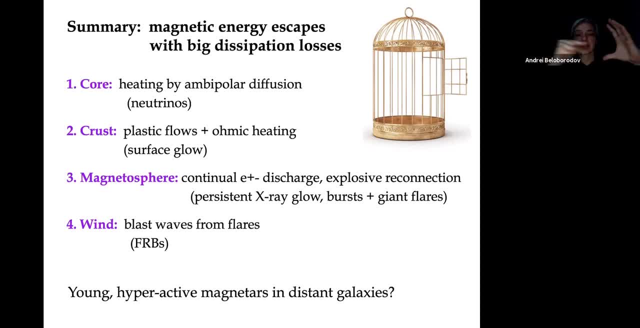 because the core is pretty much as a thermal. thermal conduction timescale across the core is very, very short. It's very good conductor, heat conductor, And so once you switch off direct OCA cooling in this massive star, you produce colder core quicker. 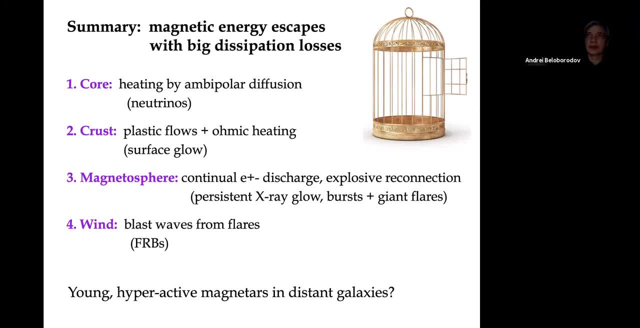 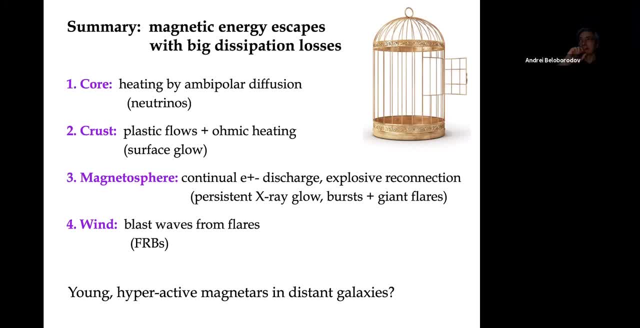 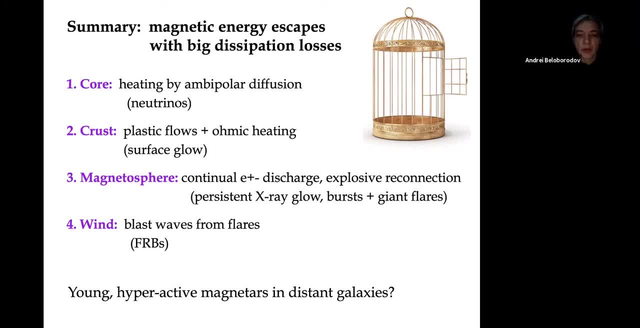 but hopefully with more data from fast radio bursts in particular, was this connection is completely established- cosmological fast radio bursts and magnetars. maybe we'll have more data to learn this kind of stuff phonologically. Theoretically I don't think we're in a position. 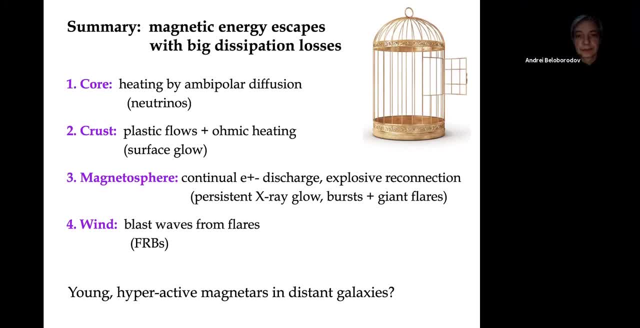 to make predictions in spite of? okay, Thank you. Okay, next question from Stephen Harris: Hi, So you mentioned at the very beginning that these flares from magnetars would cause these oscillations in the magnetar, and that could tell you something about the? 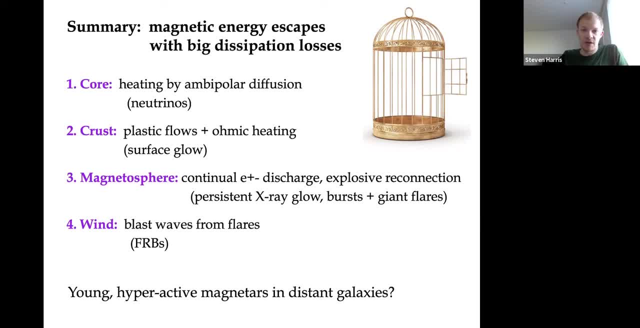 superfluidity inside of the magnetar. Do you know if they were able to determine if it was both the neutrons and the protons that were superfluid inside of the star or if it was just one or the other? Yeah, I think mostly it's just the mass that is coupled. 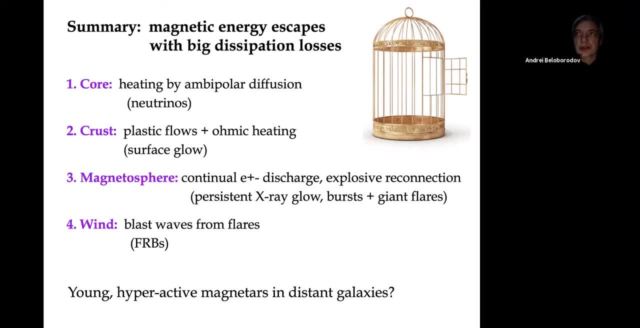 to The issue there is how much mass is tied to the oscillating field lines. So it's mostly neutrons that is an issue there. So I think you can say that neutrons are superfluid. For protons, in fact, they are not likely to be superfluid because if you look at the fields that I was 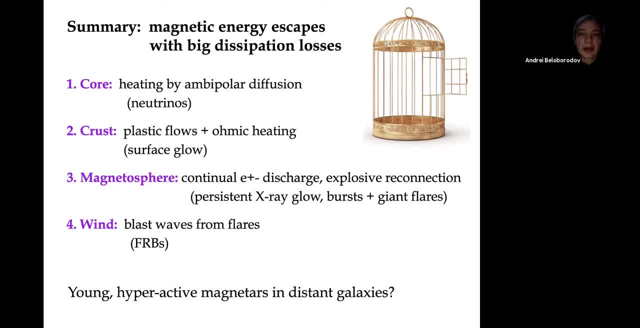 talking about 10 to the 16th Gauss. they are above the critical field that will quench proton superfluidity. Yeah, I mean it depends on density. The critical field that suppresses superconductivity depends on density And also the field doesn't have to be uniform inside the neutron star, So it's possible that. 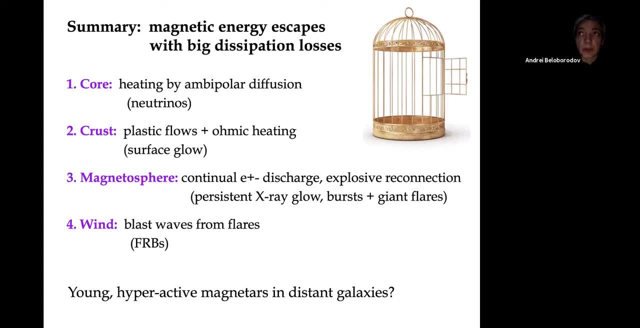 it suppresses superconductivity somewhere, but there are also normal pockets of protons, But anyway. so protons carry only like 10% or less of the mass, And so I think this, at least as far as I know. from this analysis of oscillations you can draw conclusions about. 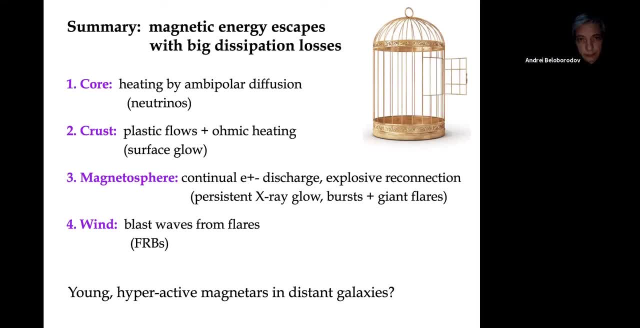 neutron superfluidity. OK, thank you. OK, any other questions? I do have a question of my own, though You didn't really mention too much about this in your talk, but somehow in the summary you kind of slipped that word: helicity of the magnetic field. that 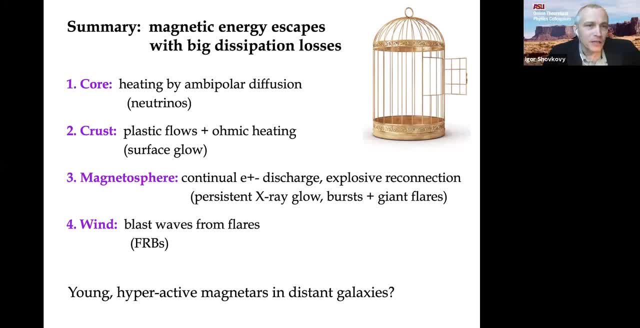 escapes, And I assume it comes basically from the fact that you have this. you call them whistlers. Sometimes people are calling them whistlers, but they're not whistlers, They're magnetic fields. Sometimes people are calling them helicons When they're coming out. this is basically. 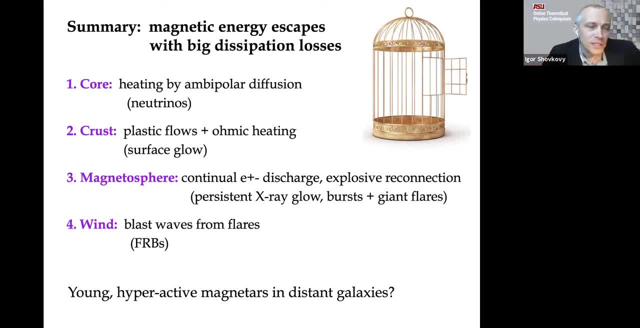 helical magnetic fields. So what's the role of helicity in this? outside, perhaps, regions of the magneton, Is the helicity a player basically? Well, helicity in this context, I think a useful kind of image of what the field is doing. 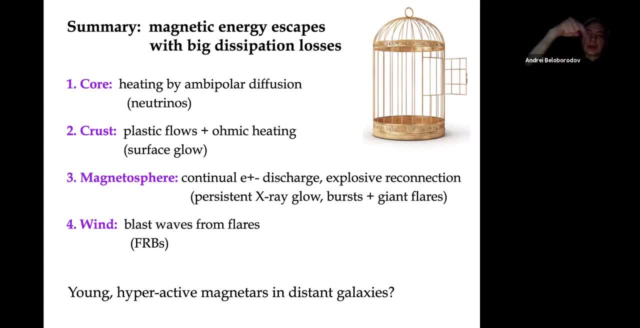 because, if you think of it as a walled-up screen, hidden, buried initially inside the core, inside the neutron star, it's likely to be, by the way, mostly throidal, because the field amplification was most likely helped by differential rotation during the neutron. 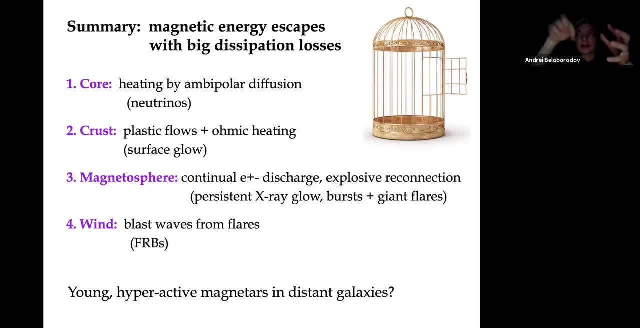 star birth. So there is a lot of ymuthal throidal field created inside the star, And so after the birth the star is in doubt wound up field. It's like his brain which would like to escape. 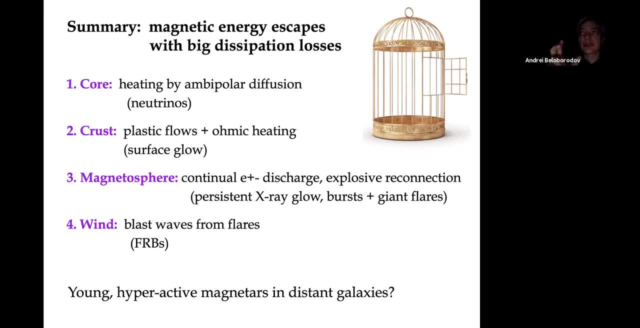 you know, just relax and get out. And so this, this helicity, tries to escape. That's how, in the simplest picture you have, when the field succeeds to unwind a little bit, you pass this winding from inside the star to the exterior of the star. 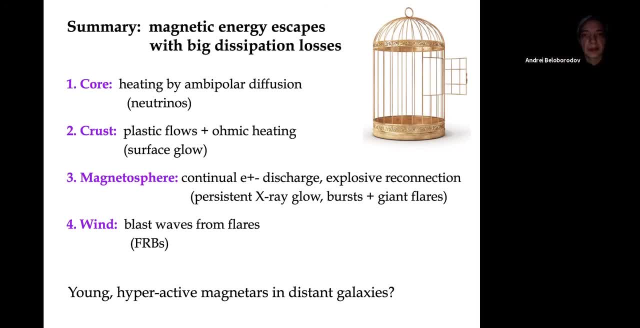 That's what the helicity transfer process that I made. And once it ends up in the magnetosphere, then you have a little resistor because the magnetosphere it does not easily sustain the electric current that you need to sustain this winding of the field. 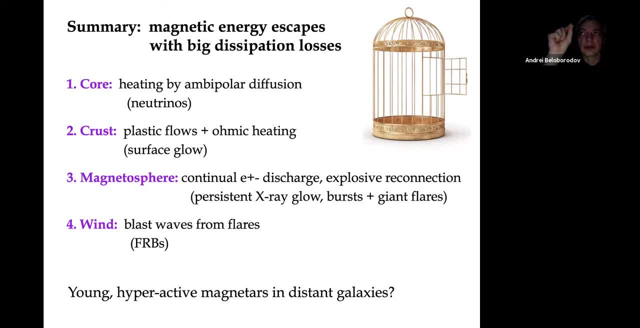 And so now you have a resistor and you have basically a dissipation. So the magnetic helicity transfer, the helicity has been transferred from very conductive material to less conductive material. You need to create electrocosm periods to keep this twist in place. 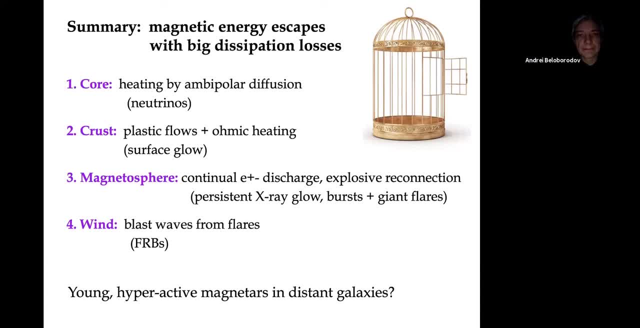 And so it has a finite lifetime. It dissipates all the time, Right, But wouldn't that imply that the emission of the photons in all the spectra will be polarized? Wouldn't you expect to see a polarized emission then? Yes, the emission is polarized. 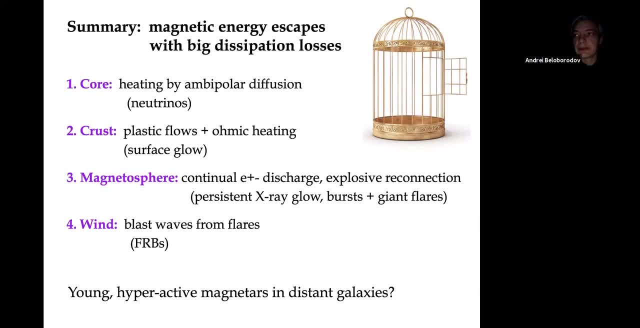 So related to the global, you know, large scale helicity in the field. but there are two polarization states of photons in this role. One has electric field, the so-called X and O mode. So one has electric field perpendicular to the K wave number of the photon. 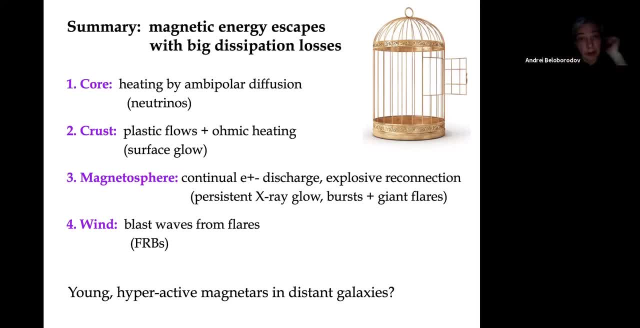 and the magnetic field, local magnet, to the same mode, And the other mode, electric field of the waves, is along that plane, a KB plane. And so, yes, so there are these eigenstates, polarized states, and you do expect the emission to be polarized. 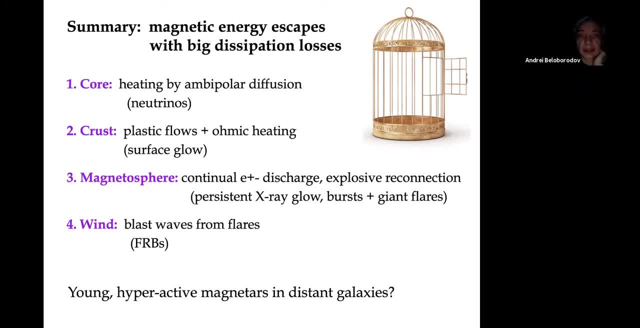 which, by the way, is being probed with soon by the polarization. We'll have polarization X-ray polarization data soon. Yeah, It depends on. of course it's going to be different depending on how you produce and where this X-ray escape, but yeah, 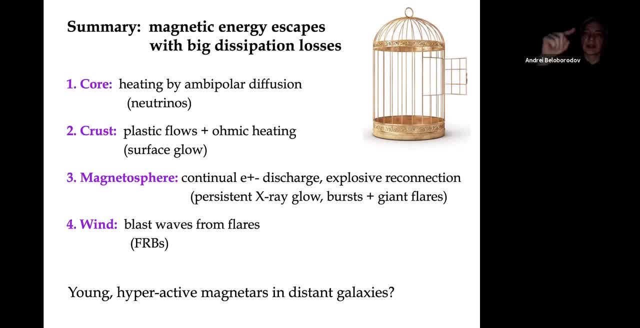 So the polarization state it should automatically tracks as the photon propagates through the magnetosphere and at some point decouples and it leaves polarization. So the polarization imprint on the observed spectrum. Yeah, Right, right, I see Very interesting. Any other questions from the audience? 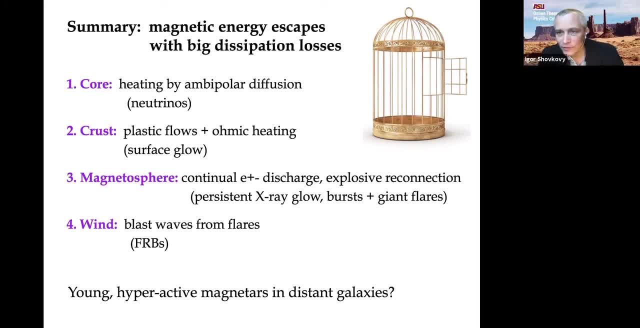 I do have another question I want to ask, but I don't want to just take my own questions. When you were talking this about the ambipolar diffusion, primarily you were talking about the interaction between protons that carry current and neutrons that basically have. 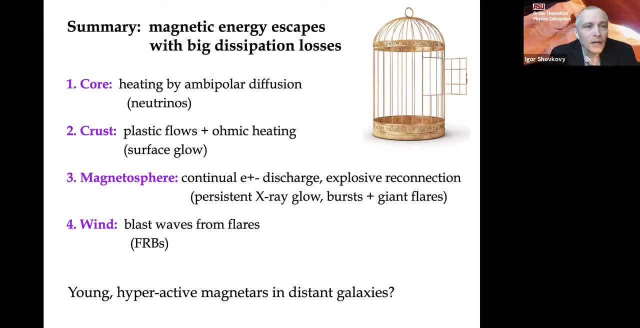 well, carry the moment of inertia. but what about the electrons? They should be carrying the current and I assume they will be scattering of protons because they are moving in the opposite direction. There should be basically some diffusion there as well. No, Yeah? 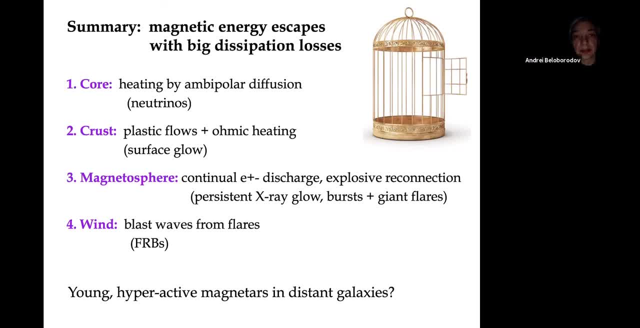 The densities are so high- electron density in the code, So density is 10 to the, let's say, 14 grams per centimeter cubed three times 10 to the 14 nuclear density. So yes, electrons are a small fraction of the protons. 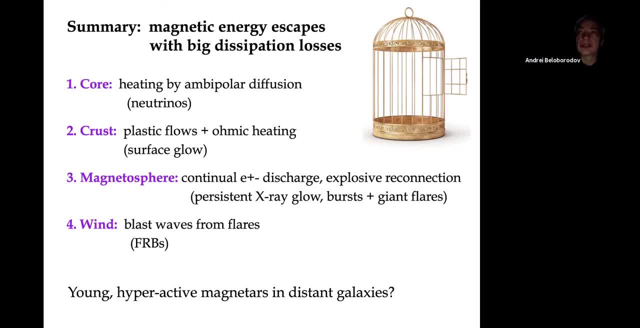 like 10%, but still there's huge number density. So to sustain the electric current that supports that magnetic field, the drift speed of electrons is tiny with respect to protons. So in the core these kind of effects in particular the whole effect that I talked about in the cross, 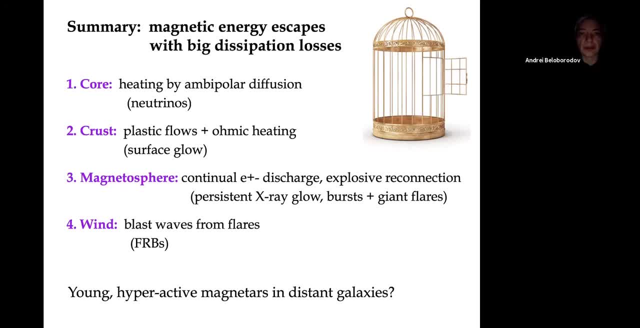 in principle it also exists in the core, because electrons are drifting with respect to protons, but because of of high densities in the core, This effect is small. I mean, the drips are not really important, I see. So it's kind of on the contrary.